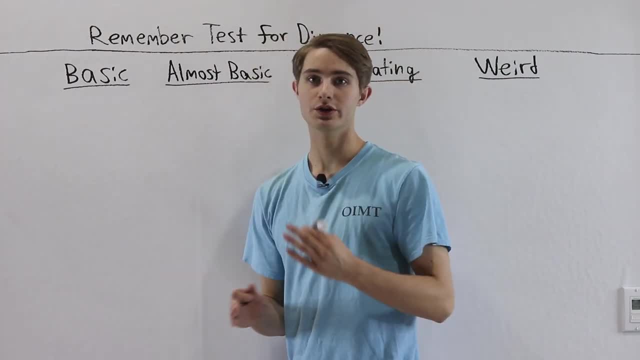 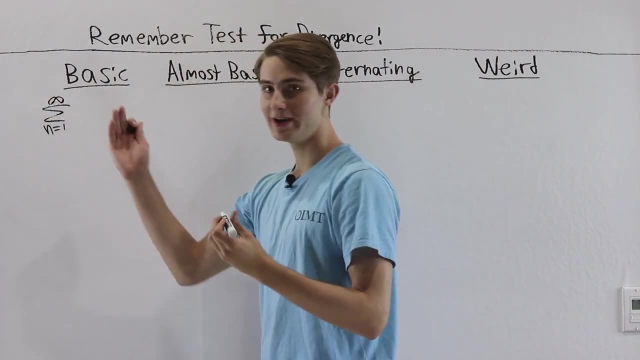 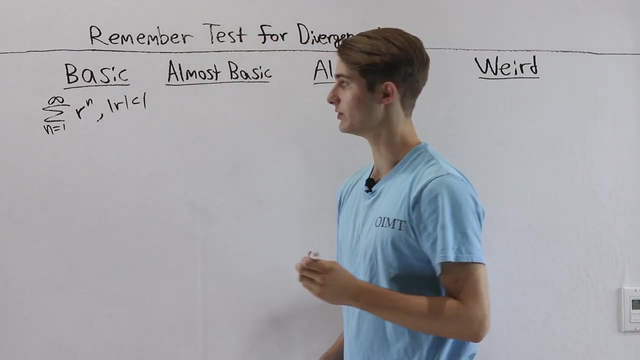 category. This is talking about those series that we already know whether they converge or diverge right away, And those two are going to be the geometric series. the sum from n equals 1 to infinity, of r to the n, which we know converges when the absolute value of r is less than 1,. 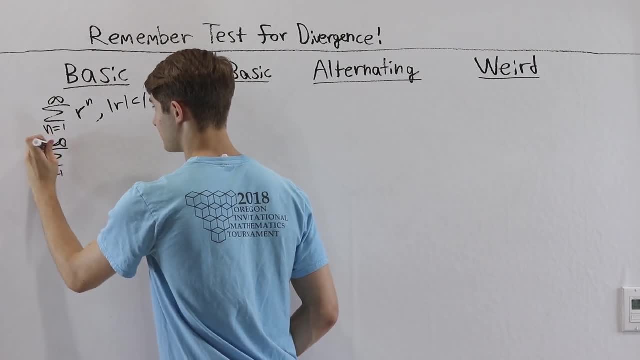 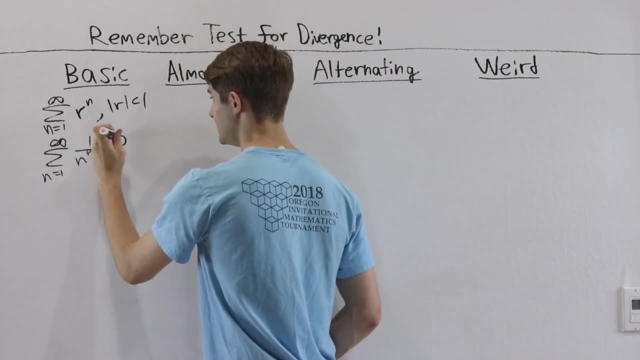 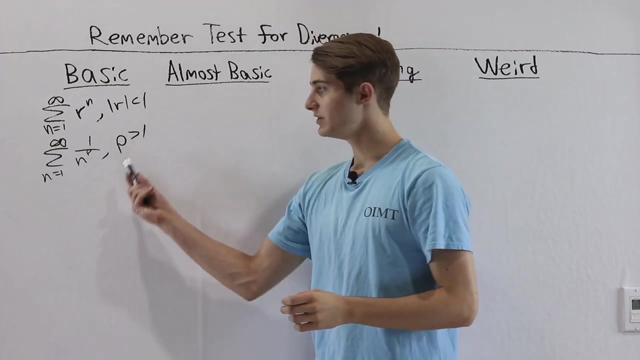 and the sum from n equals 1 to infinity of 1 over n And that's going to converge when p is greater than 1.. So this is the geometric series and the p-series formula. When we see a series that we can write in terms of one of these two things, 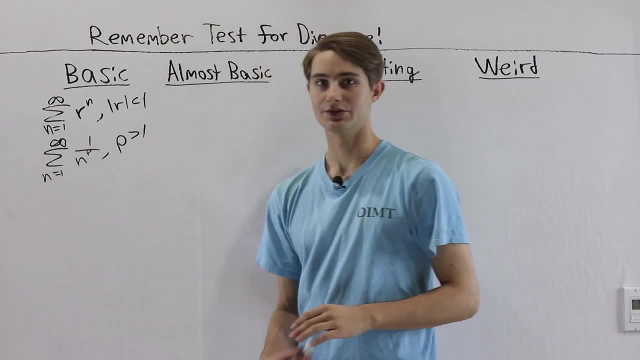 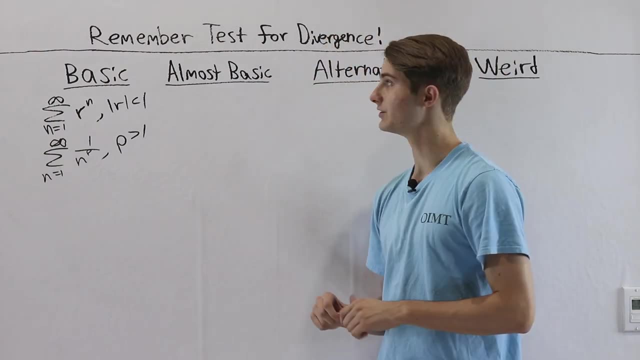 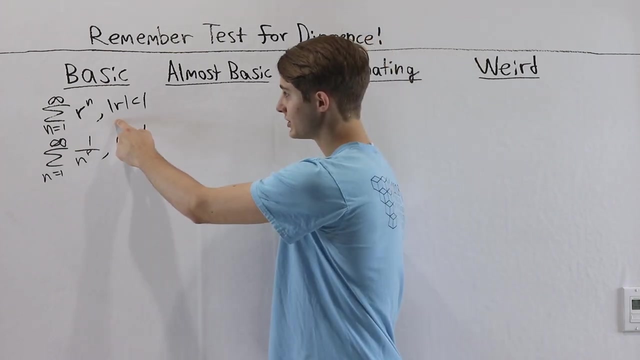 we should always do that first, because we can instantly get to an answer, just like that. But these aren't the most common types of series, so let's take a look at some of the other categories. The next one is almost basic series, And these are series that are very, very close to a geometric series or a p-series. 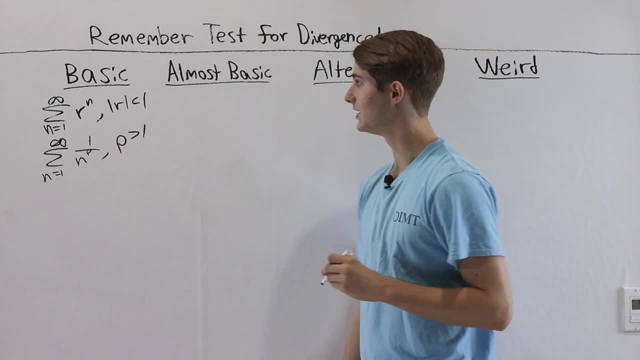 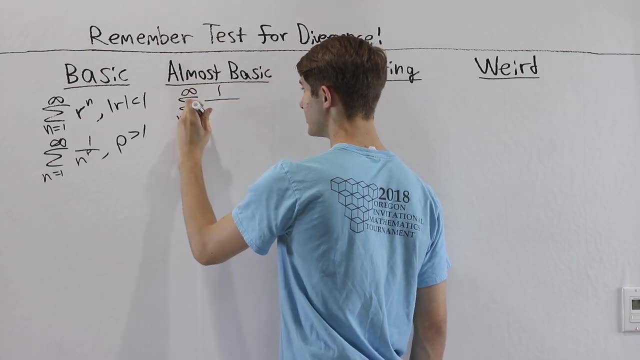 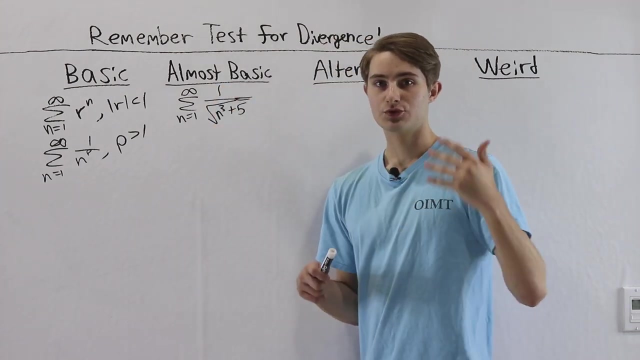 but are just not quite there. There's a little something off. For example, the sum from n equals 1 to infinity of 1 over the square root of n cubed plus 5.. So when n gets really, really, really large, notice, inside of this square root, n cubed is going to blow up. It's going to be massive. 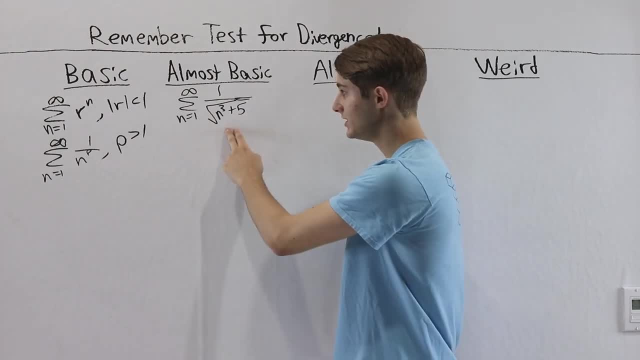 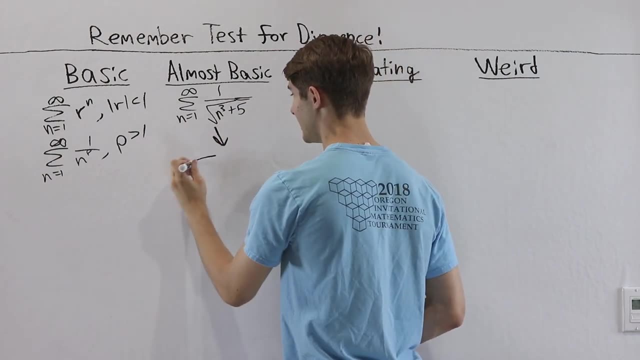 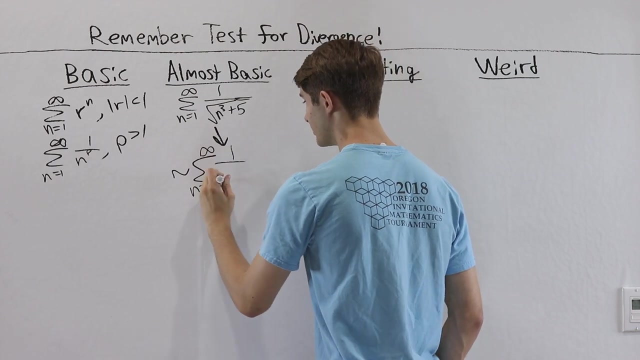 But 5 is just going to stay as 5.. So the bigger we get in this series, the less this plus 5 is going to matter. It's basically just going to be n cubed. So we can write this as, basically, the sum from n equals 1 to infinity of 1 over the square root of n cubed. 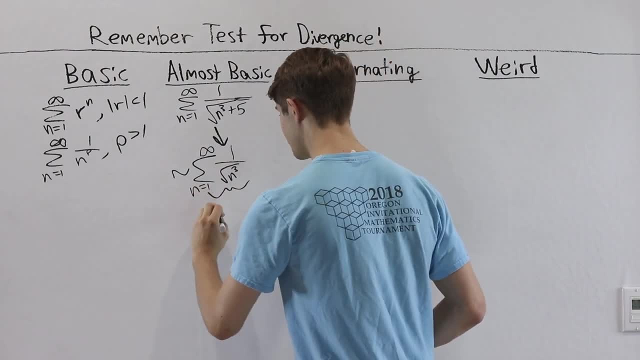 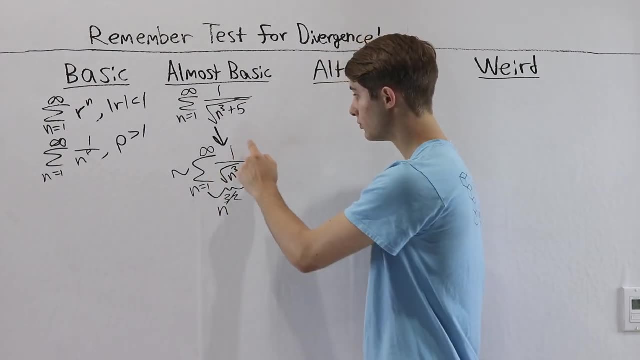 But notice that the square root of n cubed is something that we can write as n to the power of 3 halves And if we have the sum from n equals 1 to infinity, infinity of 1 over n to the 3 halves. that is a p-series and we know that it converges. 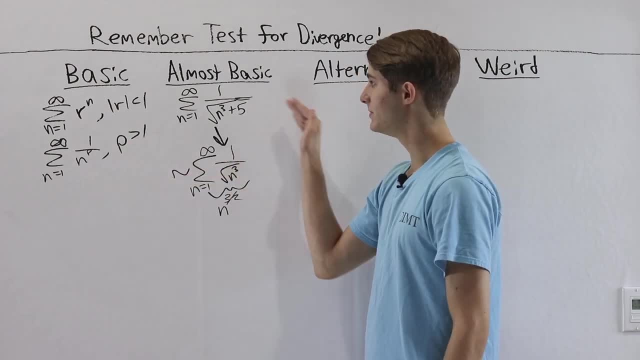 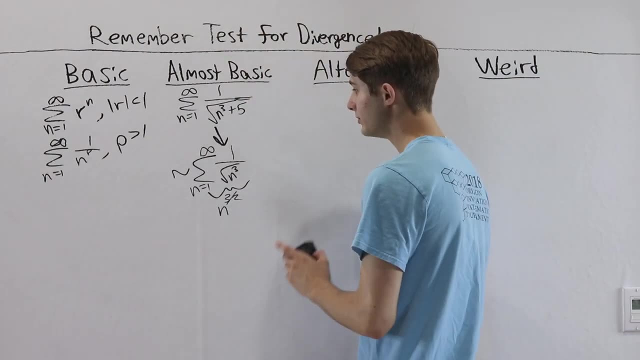 So these kinds of series where it's basically a p-series, it's basically geometric, but there's a little thing that's throwing it off. these are almost basic series, And the way that we evaluate this kind of series is always by using a comparison test. So there are two. 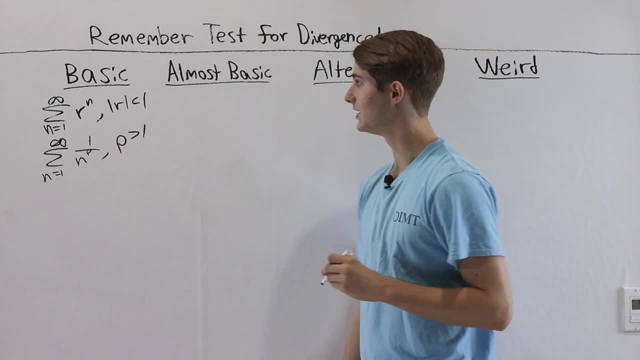 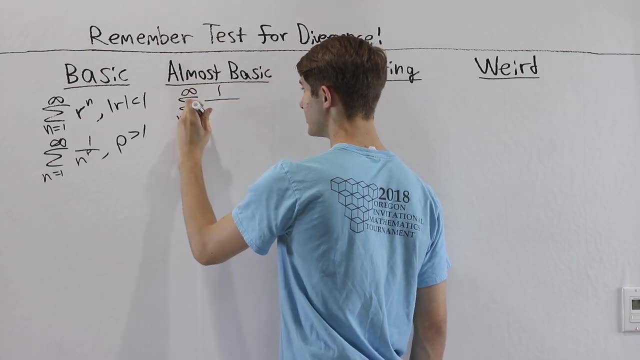 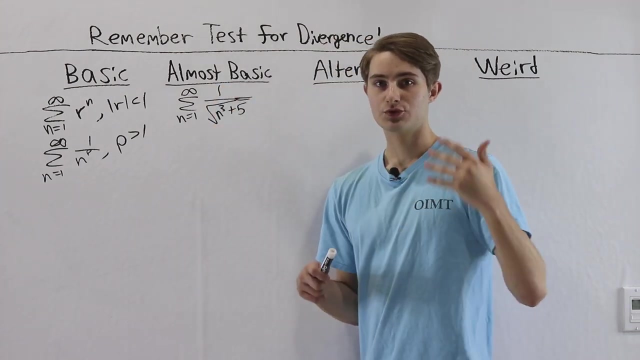 but are just not quite there. There's a little something off. For example, the sum from n equals 1 to infinity of 1 over the square root of n cubed plus 5.. So when n gets really, really, really large, notice, inside of this square root, n cubed is going to blow up. It's going to be massive. 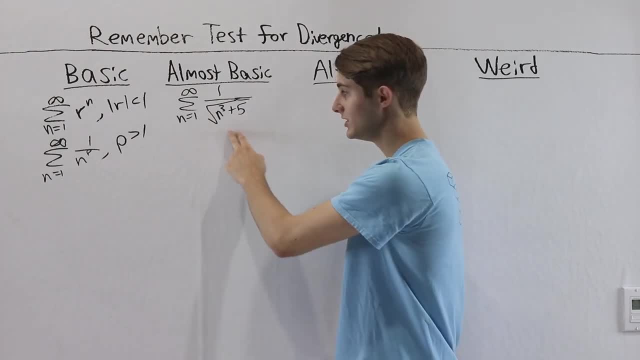 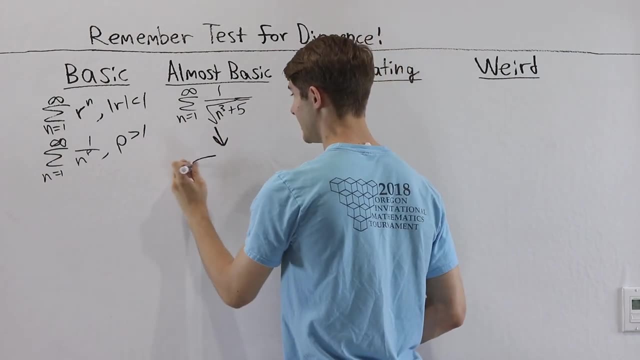 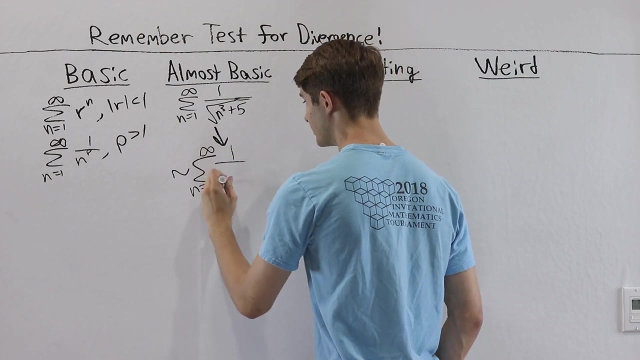 But 5 is just going to stay as 5.. So the bigger we get in this series, the less this plus 5 is going to matter. It's basically just going to be n cubed. So we can write this as, basically, the sum from n equals 1 to infinity of 1 over the square root of n cubed. But notice that the square 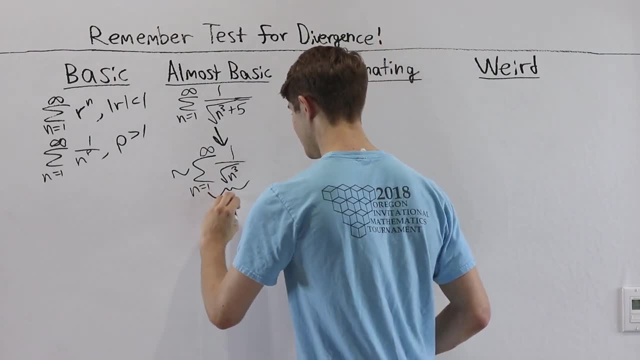 root of n cubed is something that we can write as n to the power of 3 halves, And if we have the sum from n equals 1 to infinity, that's going to be just n cubed, And the way I want to write this is: 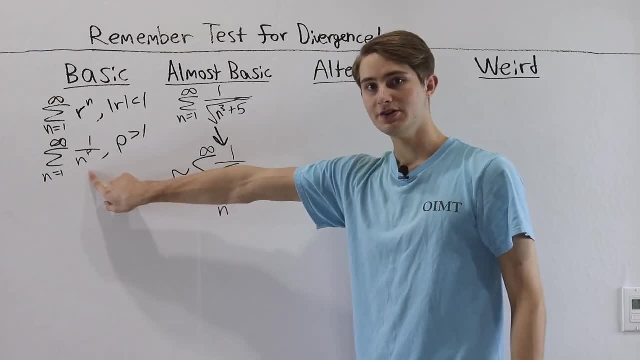 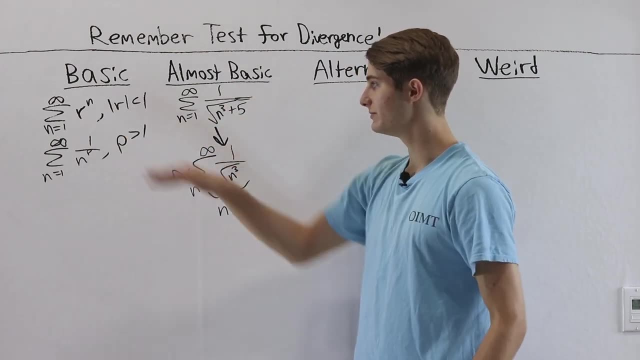 we want to connect the first two numbers to the first two numbers with the first two numbers And infinity of 1 over n to the 3 halves. that is a p-series and we know that it converges. So these kinds of series where it's basically a p-series, it's basically geometric. but there's 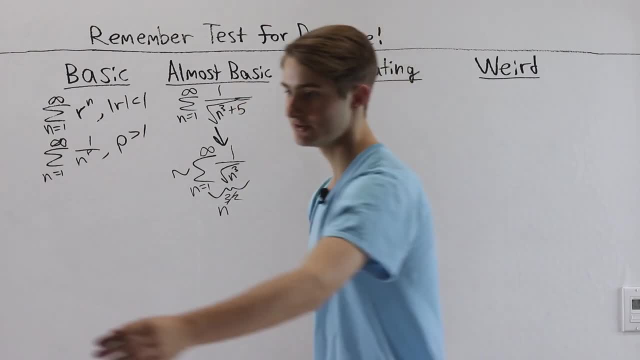 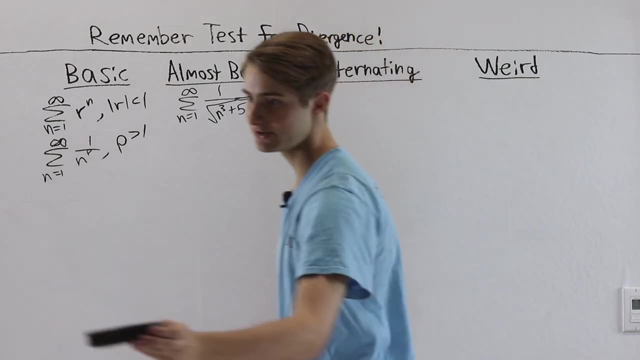 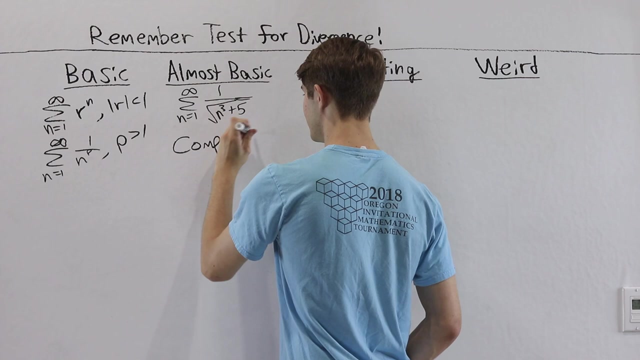 a little thing that's throwing it off. these are almost basic series, And the way that we evaluate this kind of series is always by using a comparison test. So there are two comparison tests, which are the standard comparison test or the direct comparison test, and the 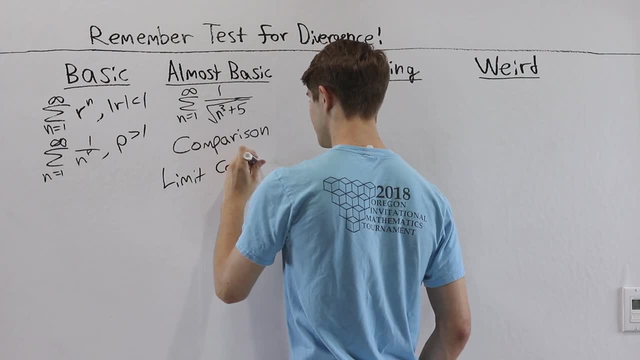 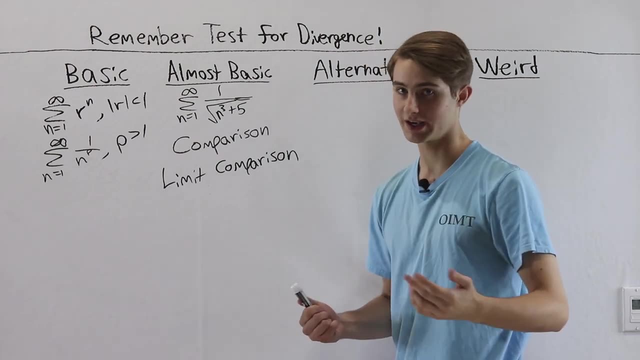 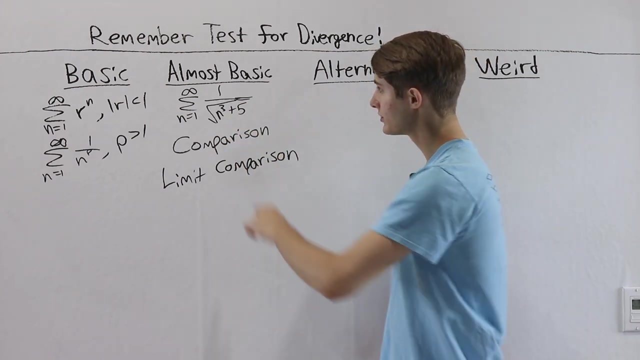 limit comparison test, And it doesn't generally matter which one we use. the limit comparison test will usually work in more of the cases, but sometimes we can get away with the comparison test as well. So in the case of this series here, notice on the bottom n cubed plus 5,. 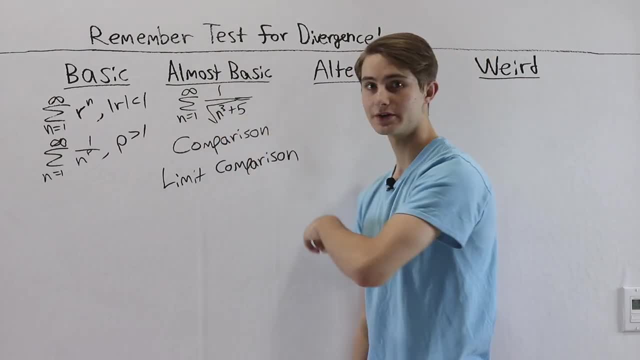 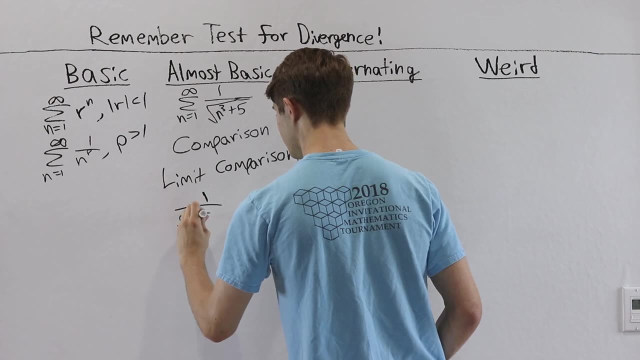 that's always going to be bigger than n cubed, And if we have something bigger in the denominator, that's going to make our results smaller. So we know that 1 over the square root of n cubed plus 5, that's always going to be. 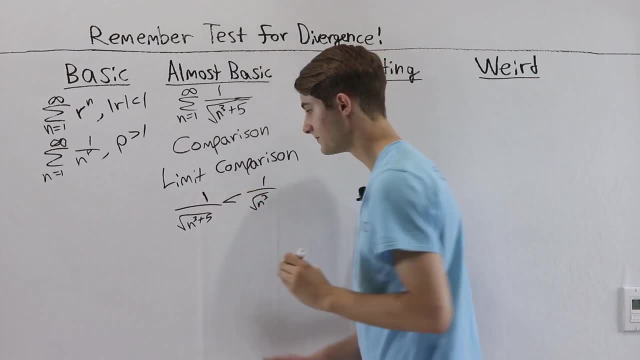 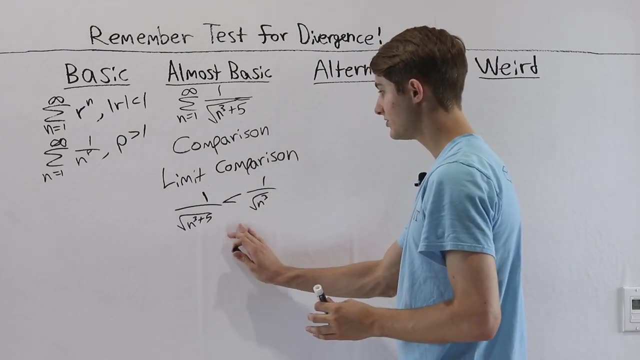 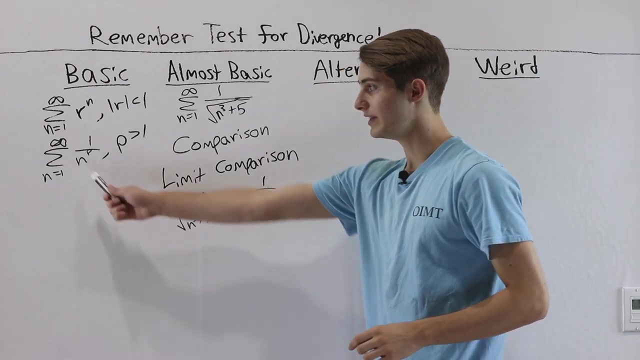 less than 1 over the square root of n cubed. Of course, on an exam we'll have to prove this more rigorously, but this is the general reasoning that we need. Once we get to this, we can use the direct comparison test to say: well, the sum of 1 over the square root of n cubed. 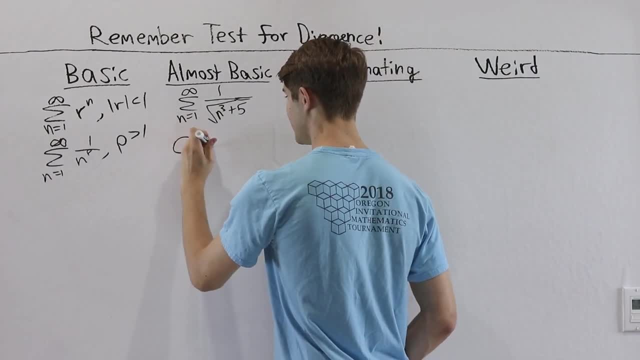 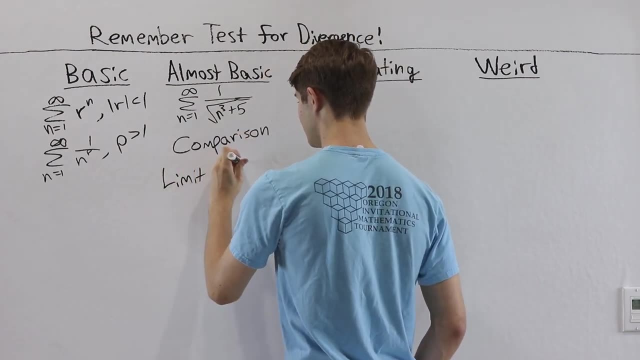 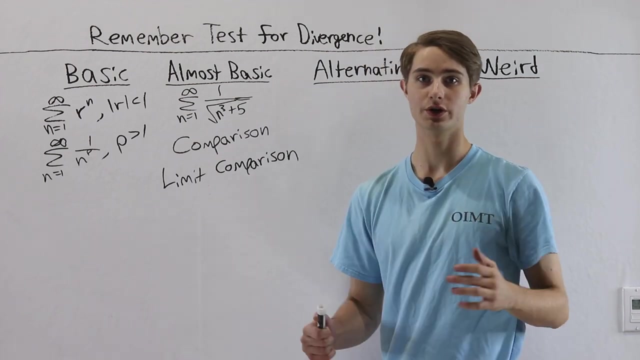 comparison tests, which are the standard comparison test or the direct comparison test and the limit comparison test, And it doesn't generally matter which one we use. the limit comparison test will usually work in more of the cases, but sometimes we can get away with the comparison. 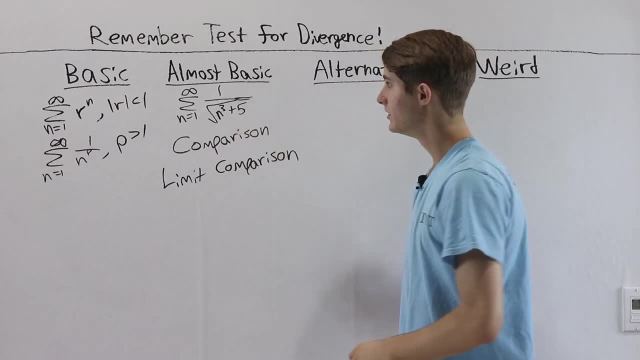 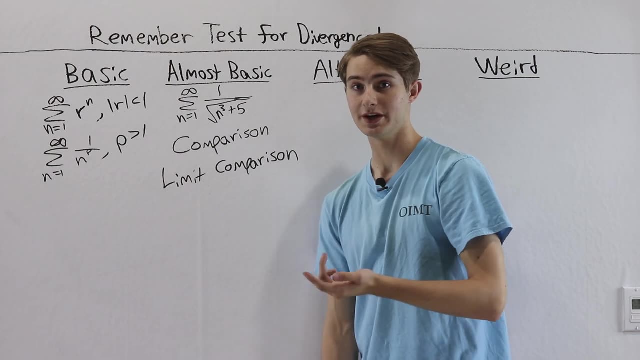 test as well. So in the case of this series here- notice on the bottom n cubed plus 5, that's always going to be bigger than n cubed, And if we have something bigger in the denominator that's going to make our results smaller. 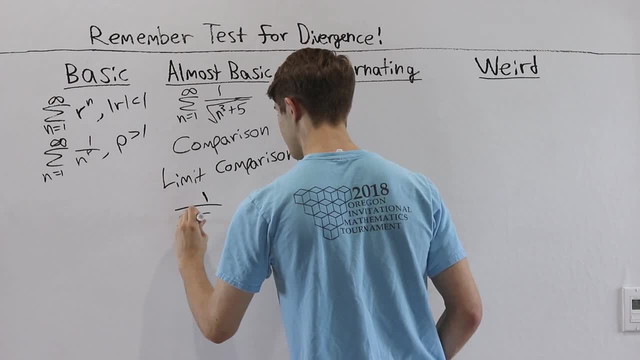 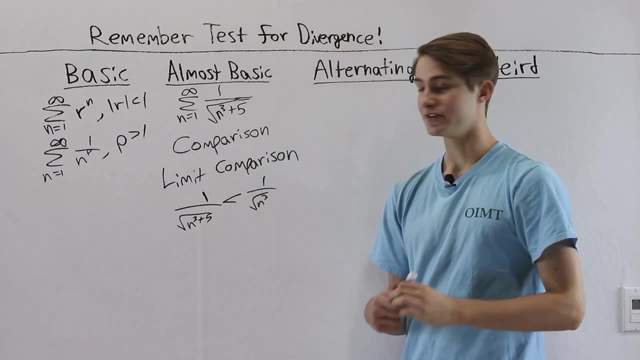 So we know that 1 over the square root of n cubed plus 5, that's always going to be less than 1 over the square root of n cubed. Of course, on an exam we'll have to prove this more rigorously, but this is the general reasoning that we need. Once we get to this, we can. 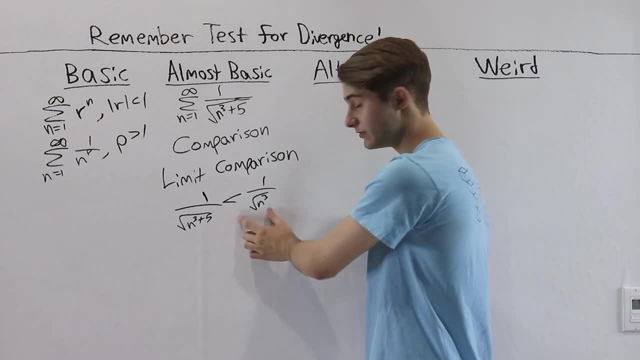 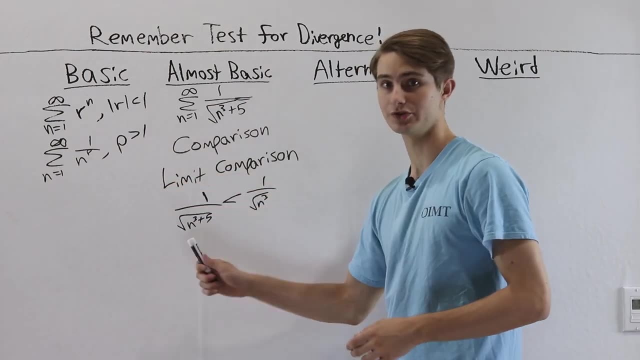 use the direct comparison test to say: well, the sum of 1 over the square root of n, cubed, that's a p-series and that can converge. Because this is less, this must also converge. So that's how we can use the. 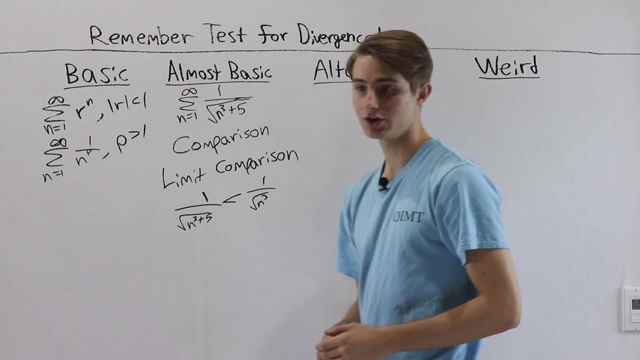 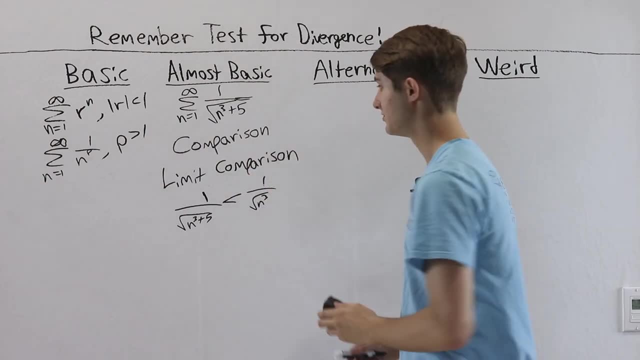 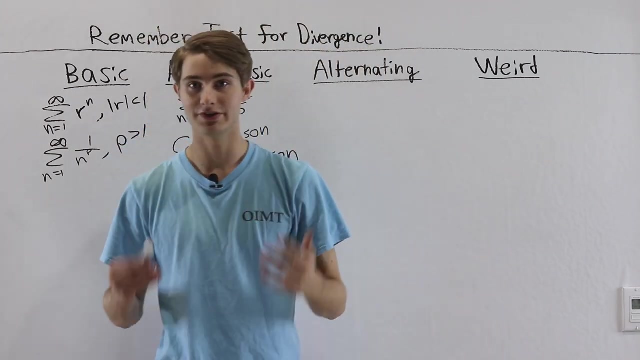 comparison test or the limit comparison test to evaluate these almost basic series, And we'll go through a few exercises at the end where we can practice identifying which type of series we're dealing with. So the next category we're going to look at is alternating series, And this is a very 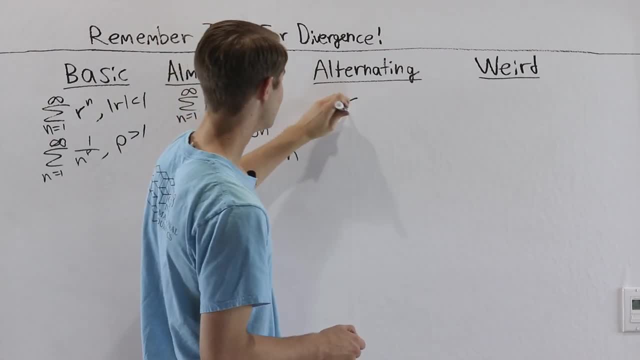 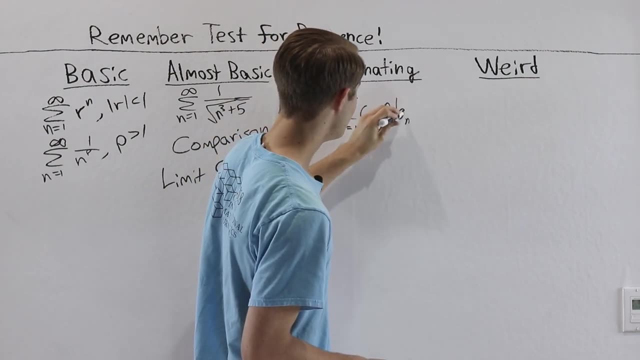 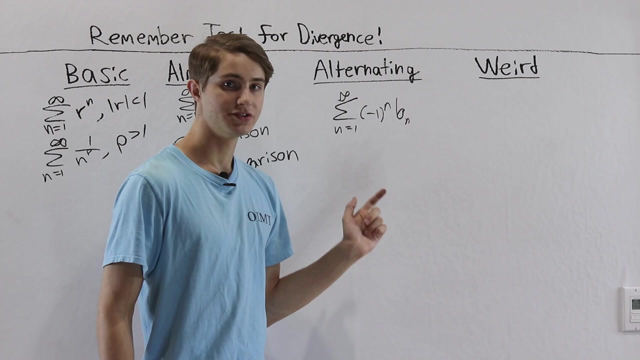 simple category. it is exactly what it sounds like. So if we have this, sum from n equals 1 to infinity of negative, 1 to the n times b sub n, where b sub n is positive, this is an alternating series and anytime we have an alternating series, it's always a good idea to try using the alternating. 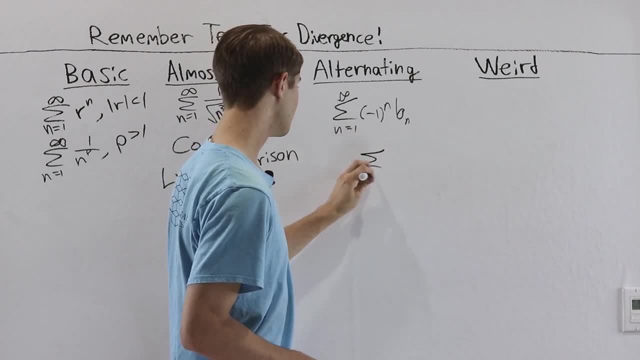 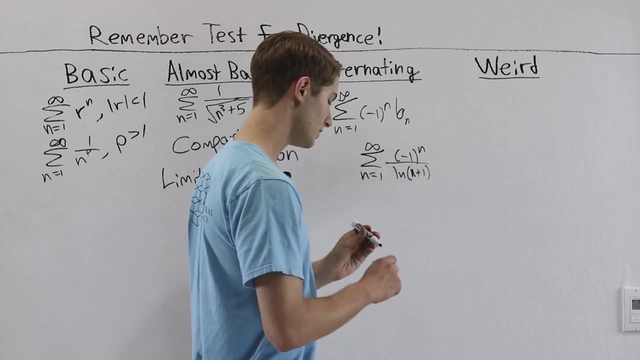 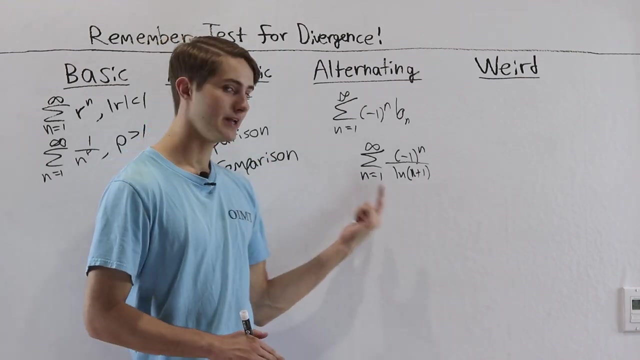 series test to see whether it converges. As an example, if we had the sum from n equals 1 to infinity, of negative 1 to the n over the natural log of n plus 1, this is an alternating series and we're going to try using the alternating series test on it. In this case we can actually prove. 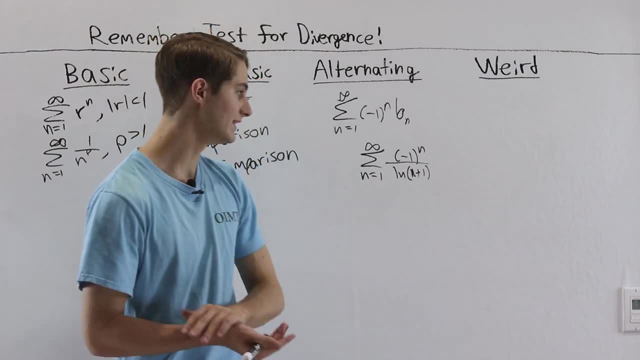 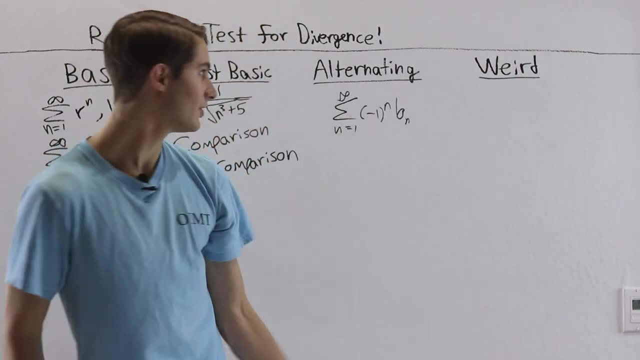 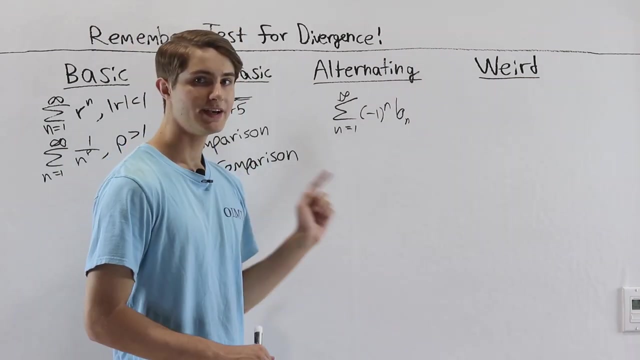 that this is an alternating series that converges by that test. So there will be some cases where an alternating series we can't prove it converges by the alternating series test. but it's always a good thing to try first. if we can pull out a negative 1 to the n. Now the last type of series. 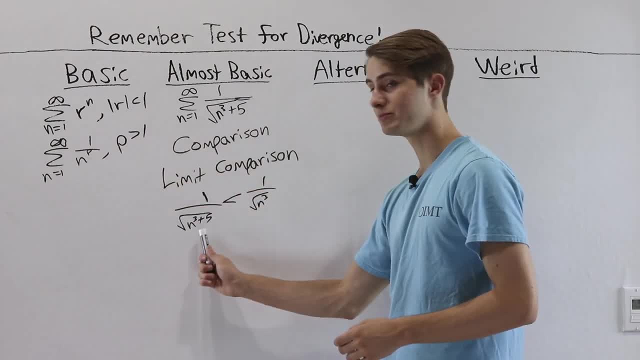 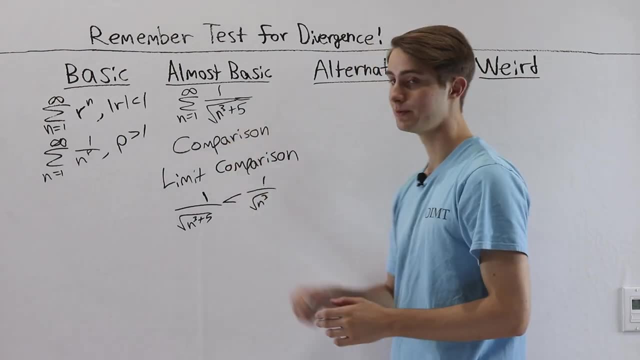 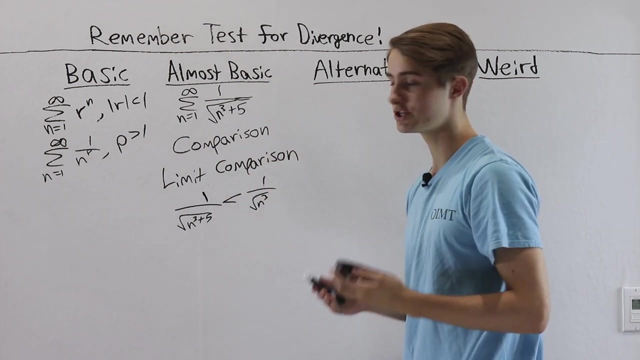 that's a p-series and that can converge, Because this is less, this must also converge. So that's how we can use the comparison test or the limit comparison test to evaluate these almost basic series, And we'll go through a few exercises at the end where we can practice identifying which type 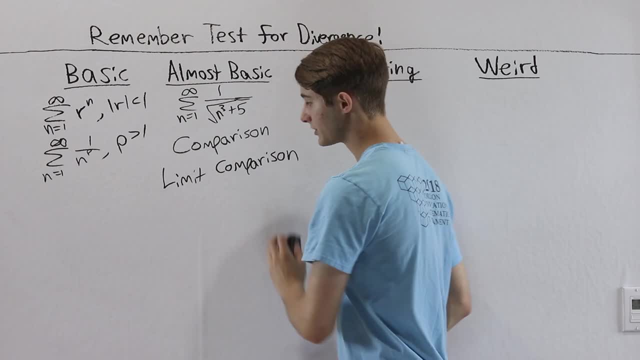 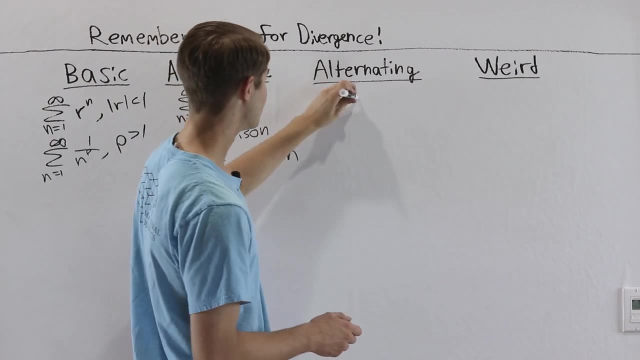 of series we're dealing with. So the next category we're going to look at is alternating series, And this is a very simple category. it is exactly what it sounds like. So, if we have the sum from n equals 1 to infinity, we're going to be looking at the p-series. 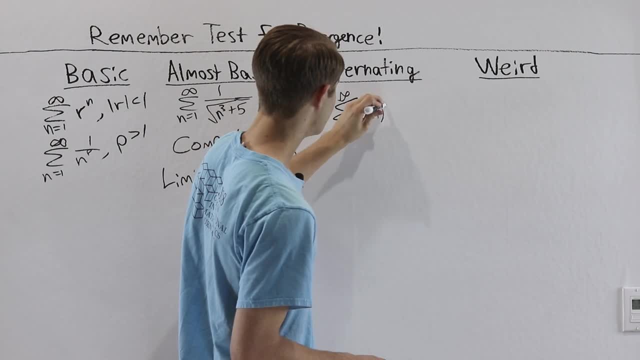 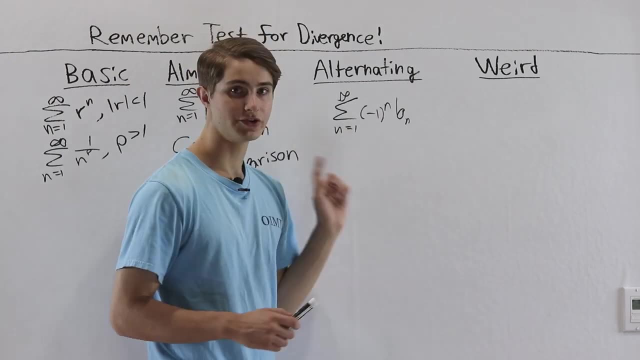 So we're going to have to figure out what the p-series is. So we have the sum from n equals 1 to infinity, and we're going to have to figure out what the p-series is. and we're going of negative 1 to the n times b sub n, where b sub n is positive. this is an alternating series. 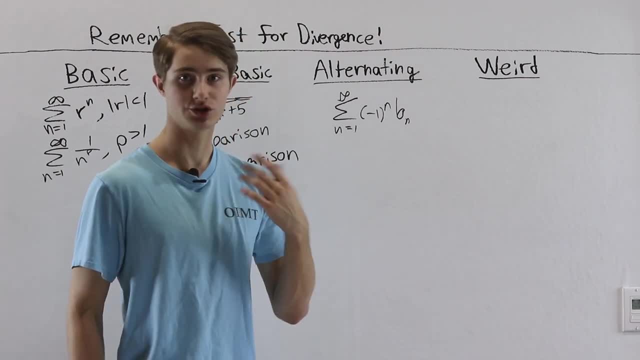 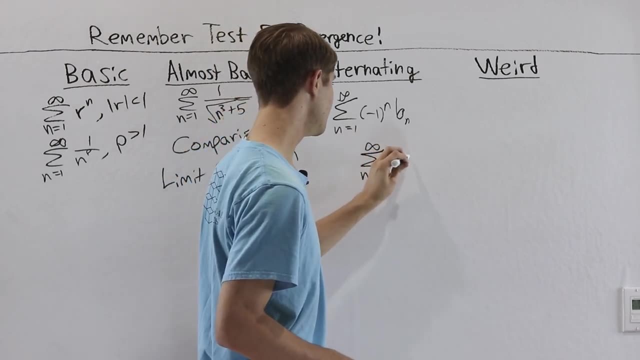 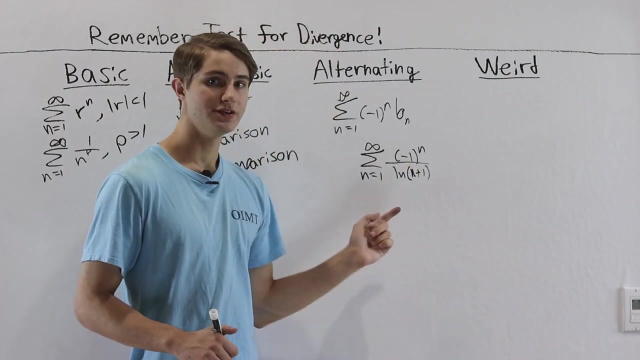 And anytime we have an alternating series, it's always a good idea to try using the alternating series test to see whether it converges. As an example, if we had the sum from n equals 1 to infinity, of negative 1 to the n over the natural log of n plus 1, this is an alternating series. 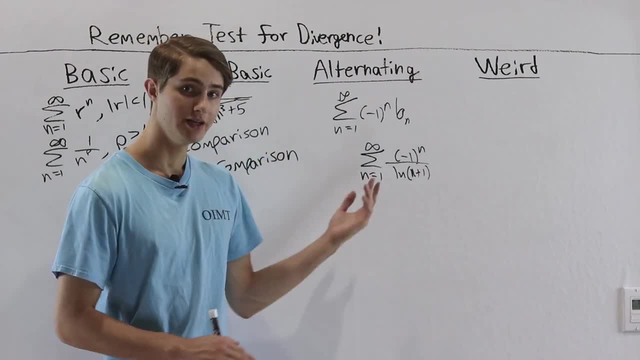 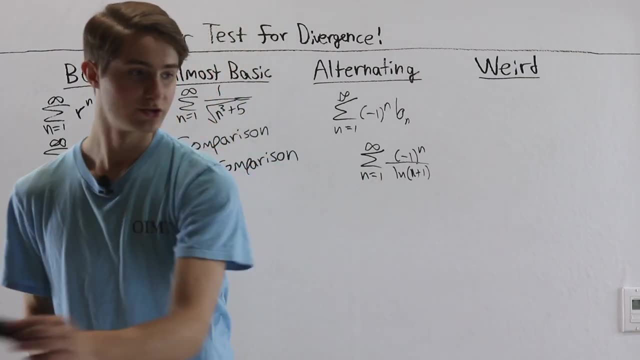 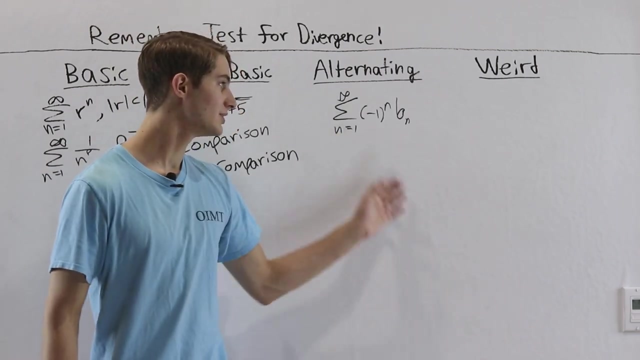 and we're going to try using the alternating series test on it. In this case we can actually prove that this is an alternating series that converges by that test. So there will be some cases where an alternating series we can't prove it converges by the alternating series test. 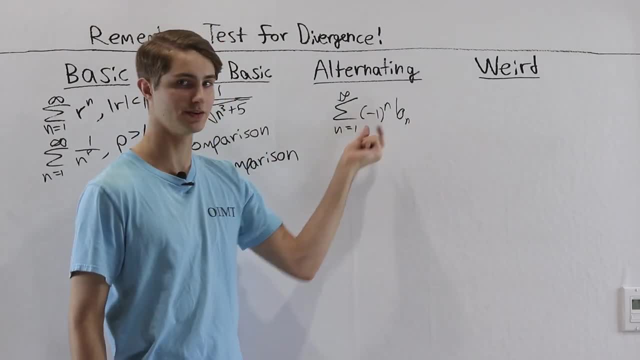 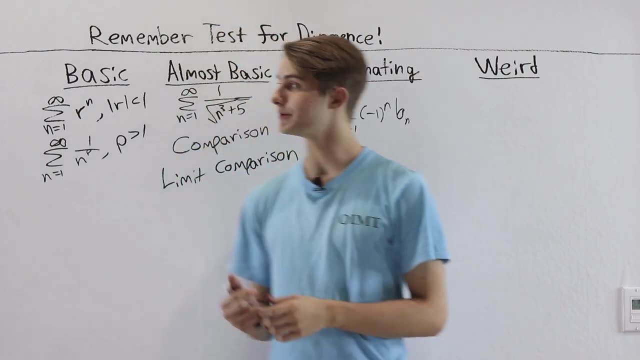 but it's always a good thing to try first if we can pull out a negative 1 to the n. Now the last type of series we're going to talk about is the weird series, and these are the series that don't really fall into any of the categories that we're going to talk about today. 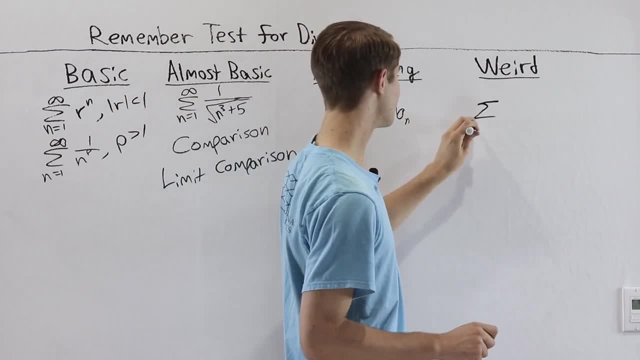 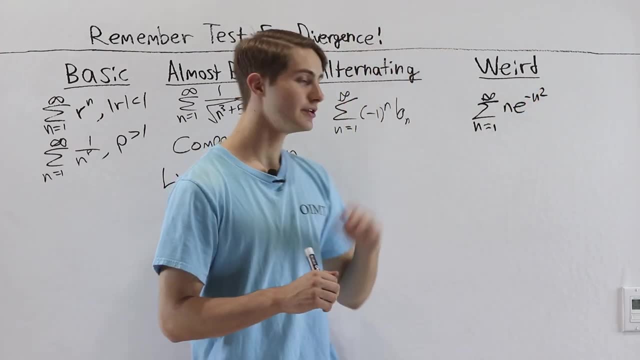 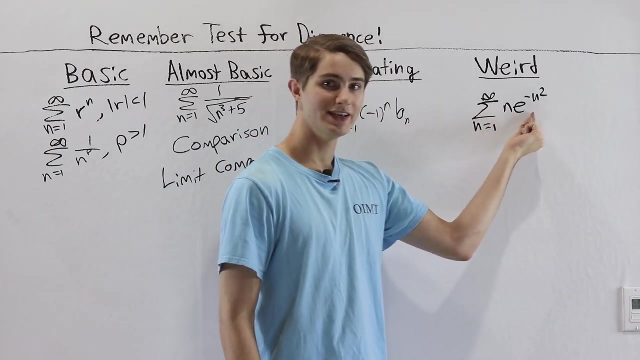 As an example, we might have the sum from n equals 1 to infinity of n times e to the negative n squared. So this clearly isn't one of our basic forms, and it's not really almost basic either, because not only do we have this n, but it's not just e to the negative n, it's e to the negative. 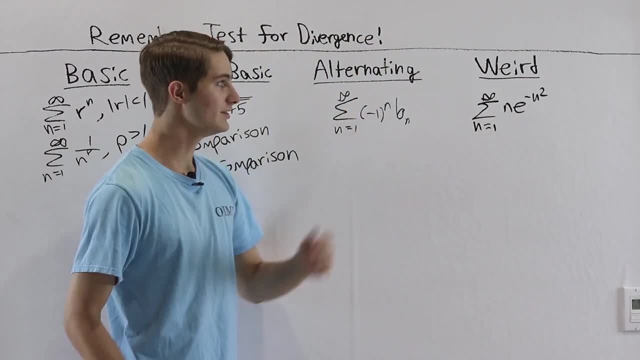 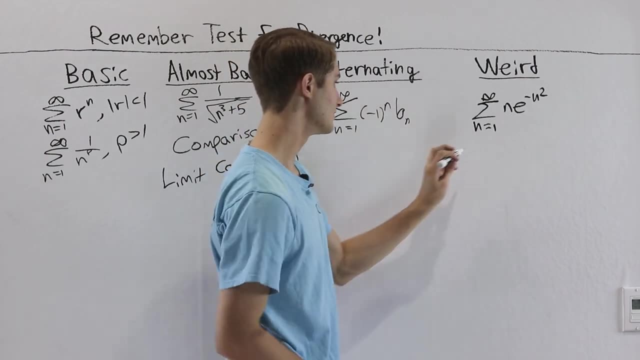 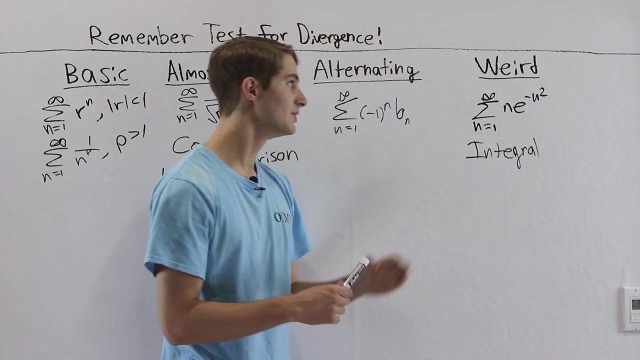 n squared, and that's just strange. It's not alternating either. So this is a case where we're going to have to use a different method, and there are two different methods that we use for weird series. The first is the integral test, and we use the integral test any time we can integrate the 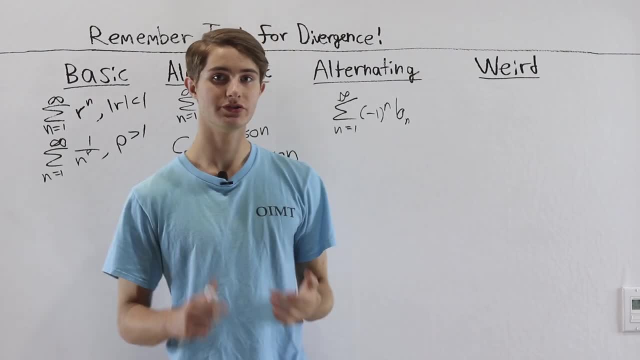 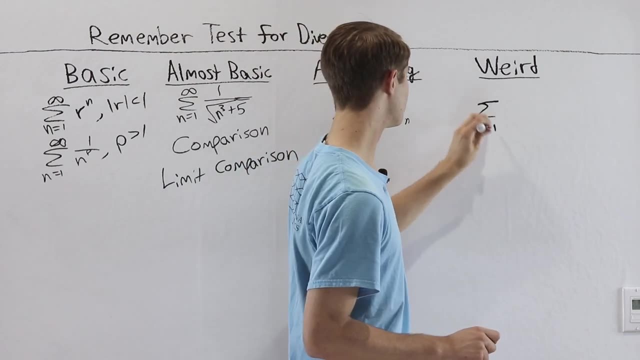 we're going to talk about is the weird series, and these are the series that don't really fall into any of the categories that we're going to talk about today. So we're going to talk about the we already talked about. As an example, we might have: the sum from n equals 1 to infinity of n. 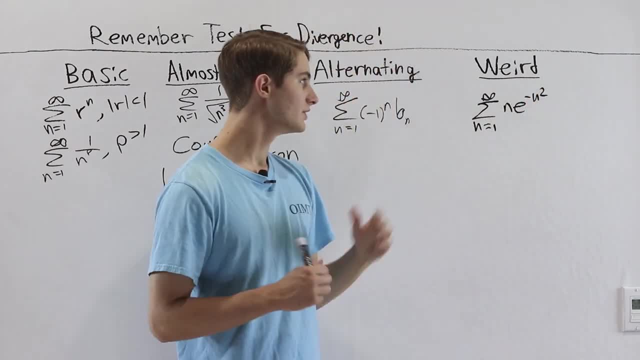 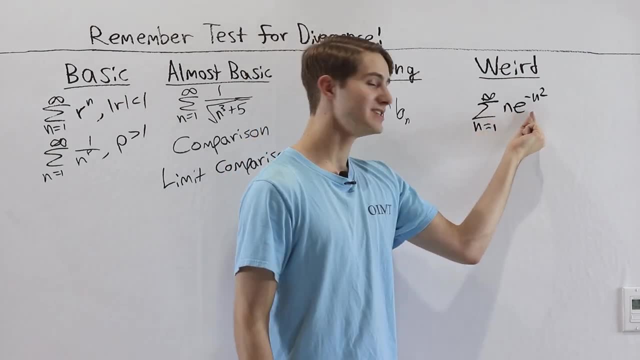 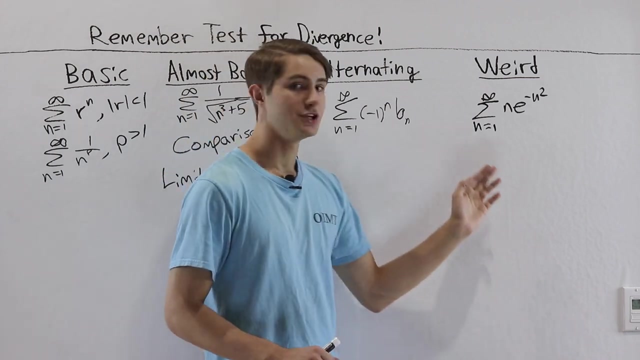 times e to the negative n squared. So this clearly isn't one of our basic forms. and it's not really almost basic either, because not only do we have this n, but it's not just e to the negative n, it's e to the negative n squared, and that's just strange. it's not alternating either. So this is a case. 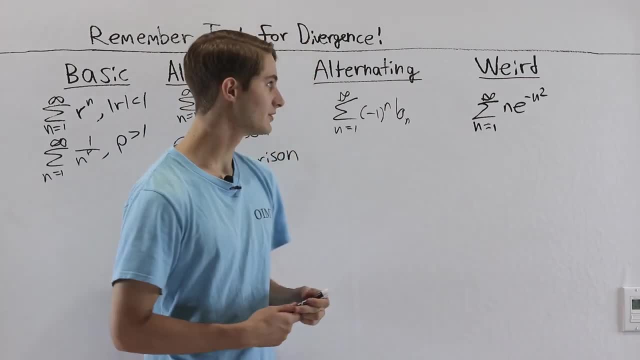 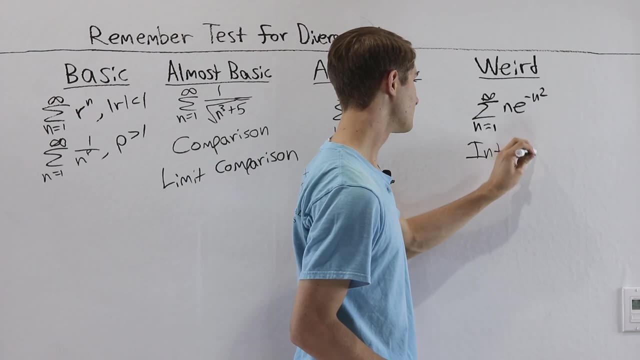 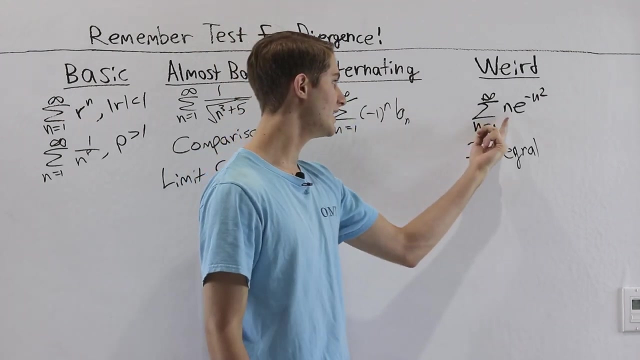 where we're going to have to use a different method, and there are two different methods that we use for weird series. The first is the integral test, and we use the integral test any time we can integrate the series. So in this case, the sum from n equals 1 to infinity, of n, e to the negative n squared. 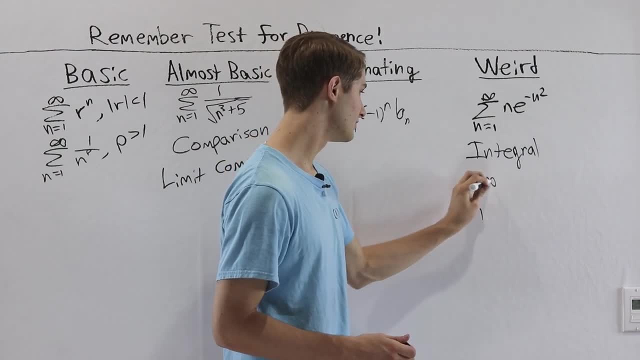 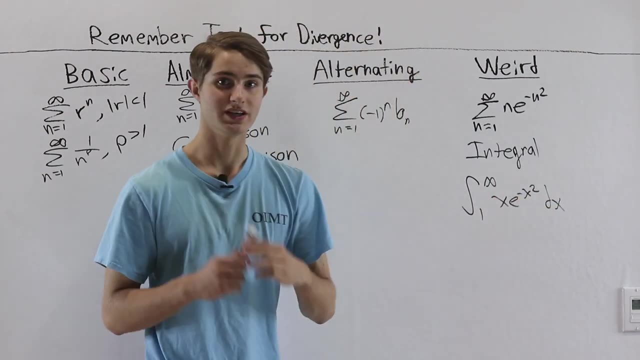 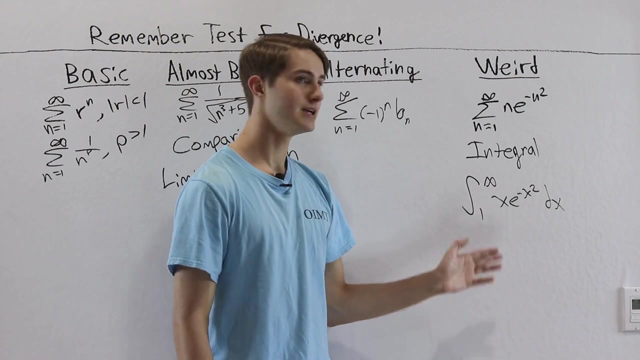 well, we are able to do the integral from 1 to infinity, of x, e to the negative x squared dx, and as long as the conditions for the integral test are satisfied, meaning it's continuous positive and decreasing over time, We are able to use the integral test for this kind of series. There's one other kind of weird series. 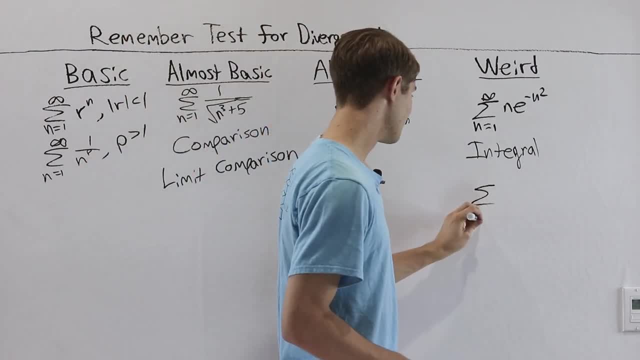 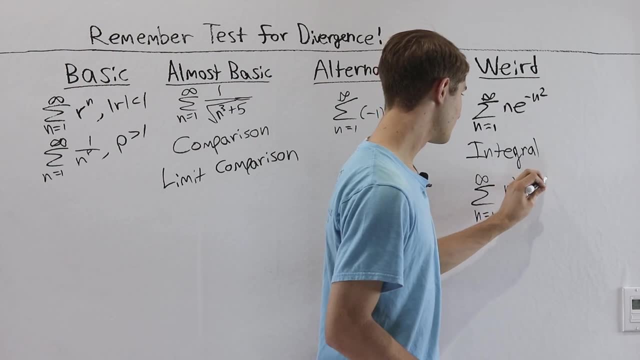 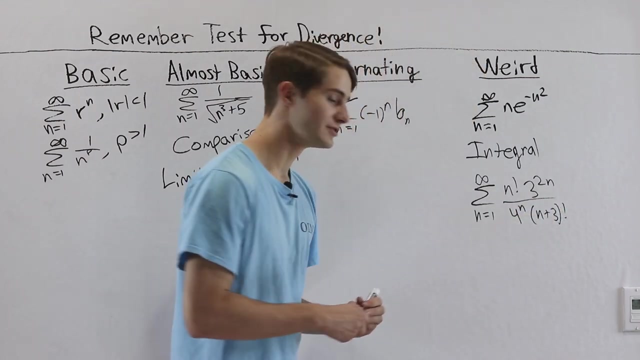 which I'll give an example of here. For example, the sum from n equals 1 to infinity of n factorial times 3 to the power of 2n over 4 to the n times n plus 3 factorial. So in this case, the important 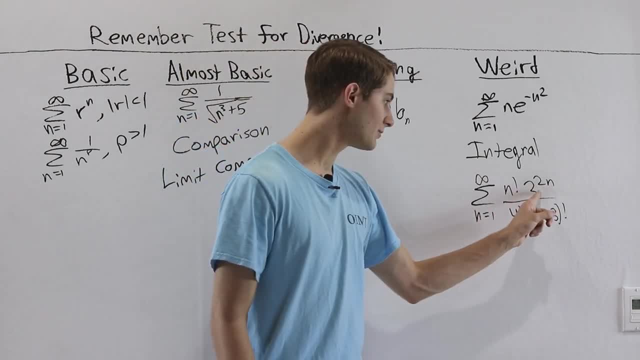 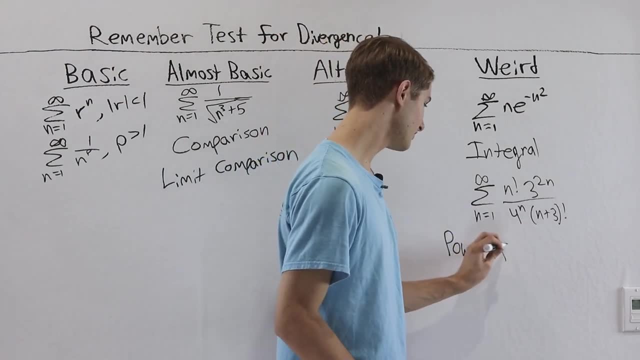 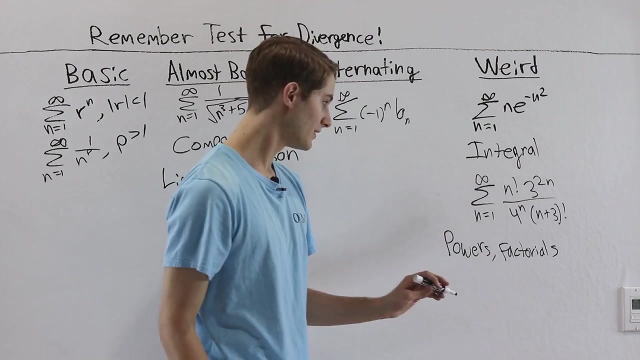 thing about these kinds of weird series is: we have power over n squared. So we have power over n squared and we have factorials. So I'll write that here: When we have powers and factorials- and when I say powers I'm talking specifically about n in the power- In that case we're going to use the ratio. 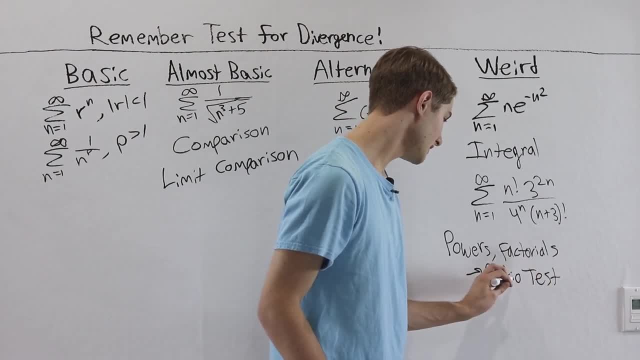 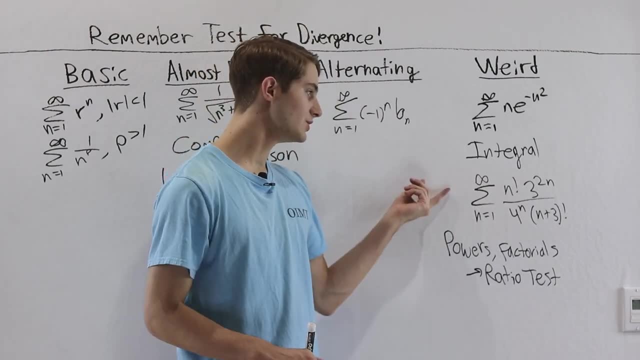 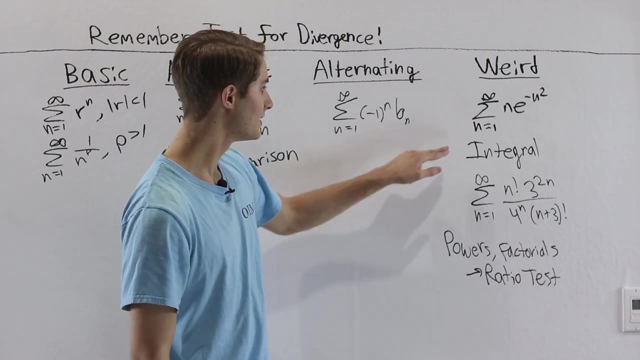 test to evaluate these. So in this case, if we use the ratio test for this series, we would be able to evaluate it to a particular number that we could use to prove that this either converges or diverges. So those are the two kinds of weird series we're talking about. 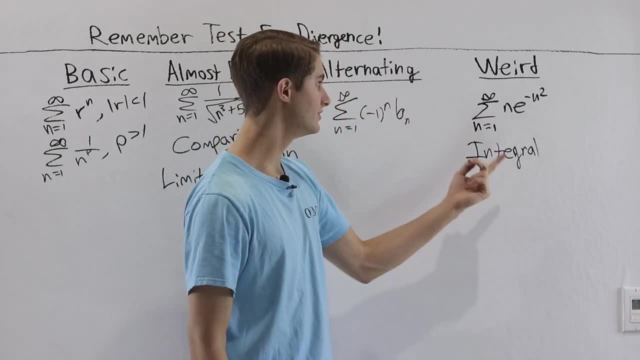 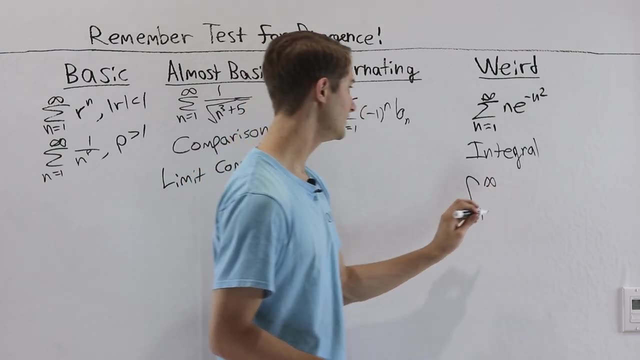 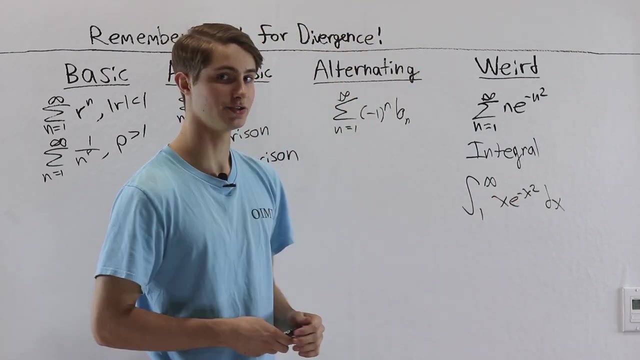 series. So in this case the sum from n equals 1 to infinity of n, e to the negative n squared. well, we are able to do the integral from 1 to infinity of x, e to the negative x squared, dx, and as long as the conditions for the integral test are satisfied, meaning it's continuous. 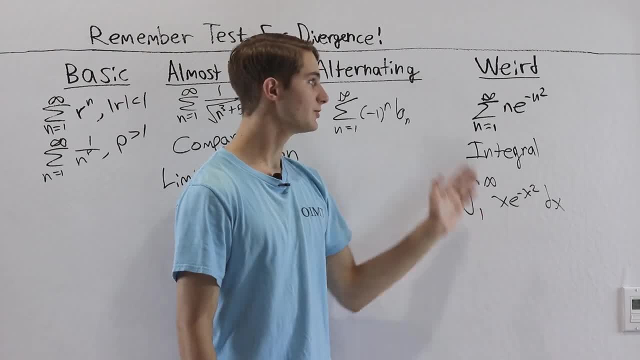 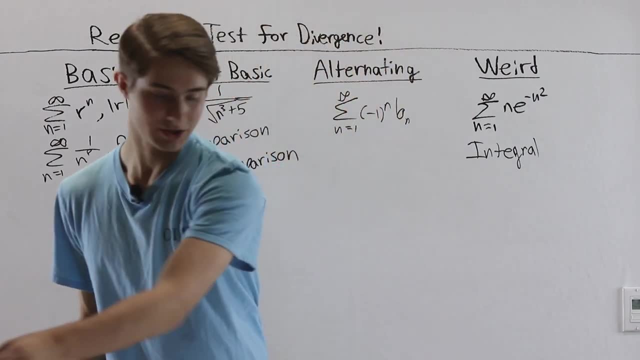 positive and decreasing over time, we are able to use the integral test for this kind of series. There's one other kind of weird series which I'll give an example of here. For example, the sum from n equals 1 to infinity. 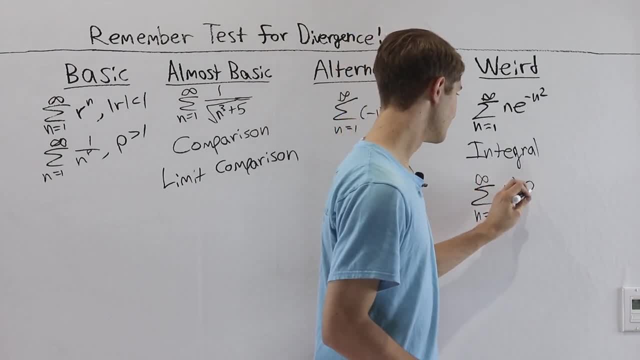 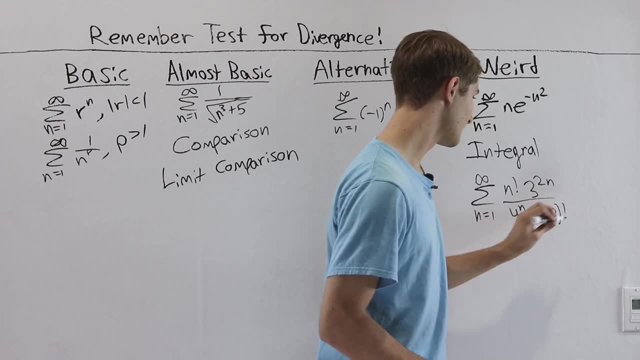 of n factorial times 3 to the power of 2n over 4 to the n times n plus 3 factorial. So in this case, the important thing about these kinds of weird series is we have a series of n factorial times 3 to the power of 2n over 4 to the n times n plus 3 factorial. 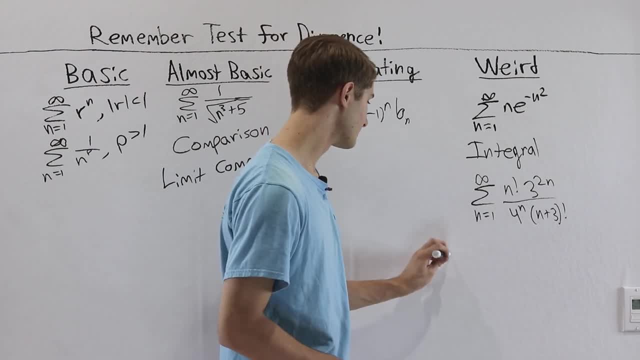 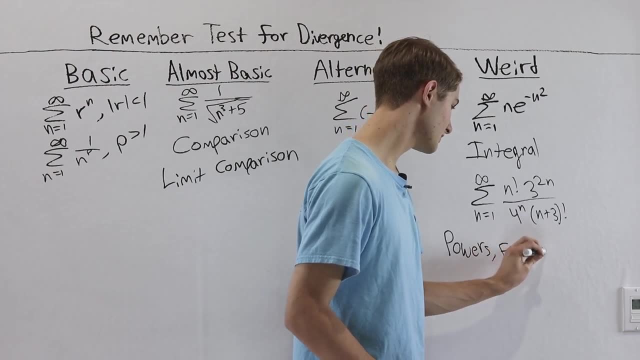 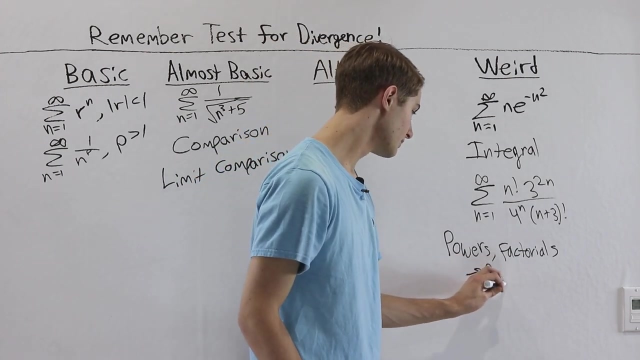 powers and we have factorials, So I'll write that here. When we have powers and factorials- and when I say powers I'm talking specifically about n in the power- in that case we're going to use the ratio test to evaluate these. So in: 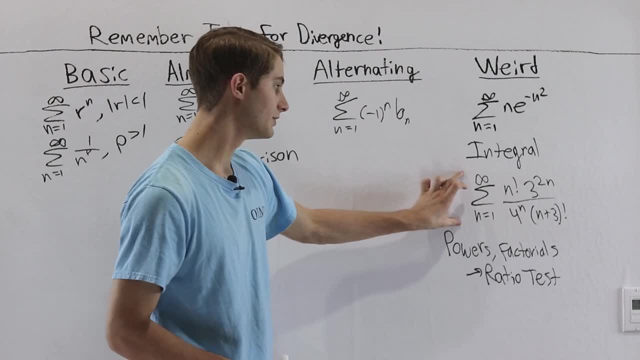 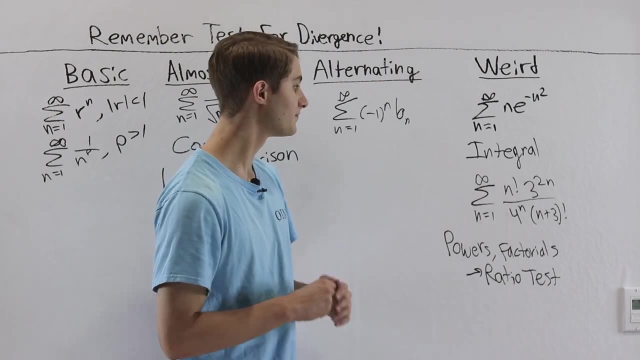 this case, if we use the ratio test for this series, we would be able to evaluate it to a particular number that we can use to prove that this either converges or diverges. So those are the two kinds of weird series we're talking about. If 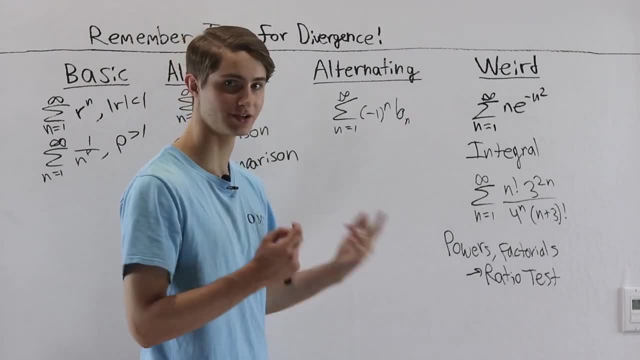 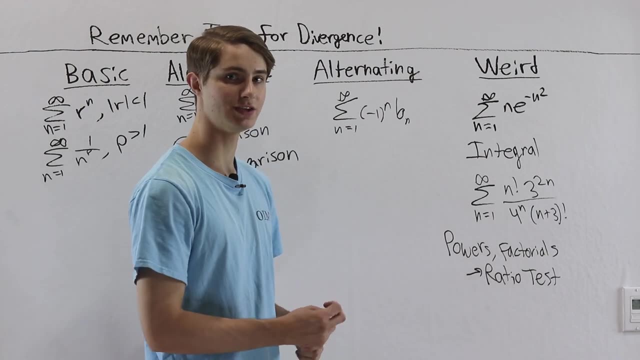 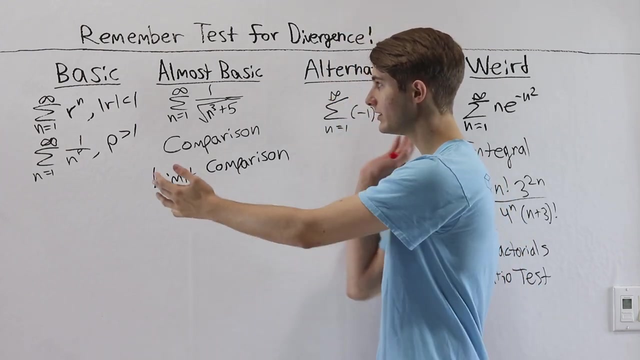 you can do the integral, do the integral test, as long as the conditions are satisfied And if we have factorials and powers flying around everywhere, that's when we're going to try the ratio test. So now that we've identified all of these categories, let's go through a few exercises where we try to figure out. 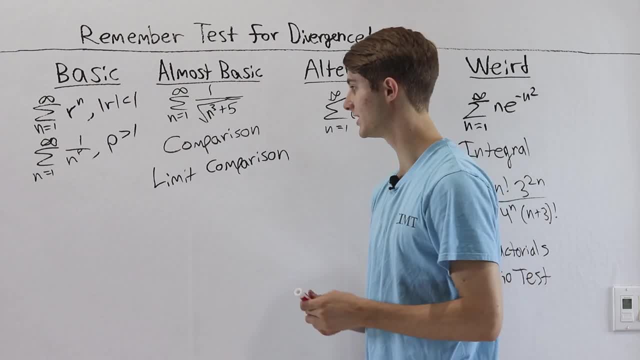 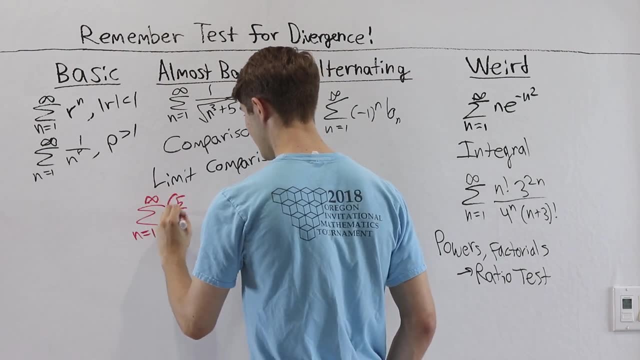 which type of series we're looking at. so we know which test to apply. Let's start out with a basic one. the sum from n equals 1 to infinity of 5 halves to the power of negative 2n. This already sort of looks. 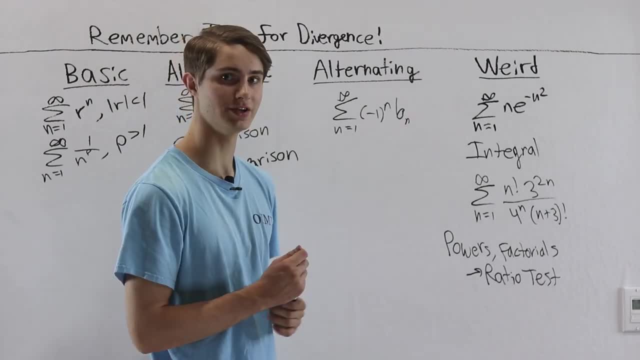 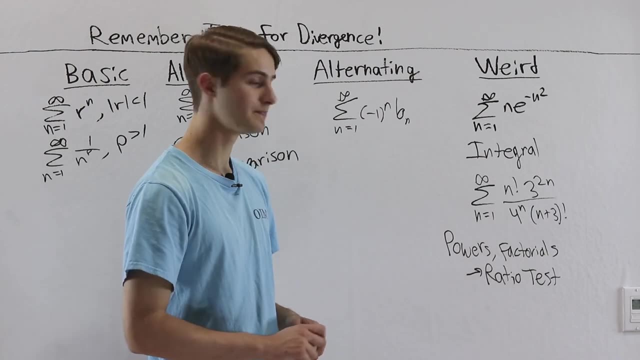 If you can do the integral, do the integral test. as long as the conditions are satisfied and if we have factorials and powers flying around everywhere, that's when we're going to try the ratio test. So now that we've identified all of these categories, let's go through a few exercises where we try to 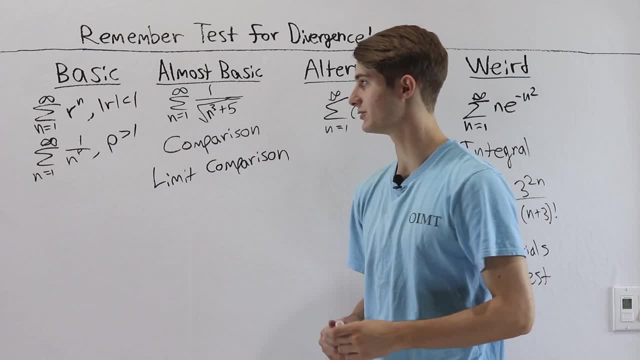 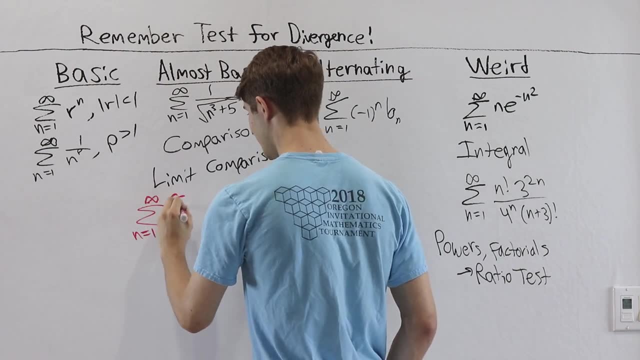 figure out which type of series we're looking at. so we know which test to apply. Let's start out with a basic one. The sum from any equation equals one to infinity of five halves to the power of negative two n. This already sort of 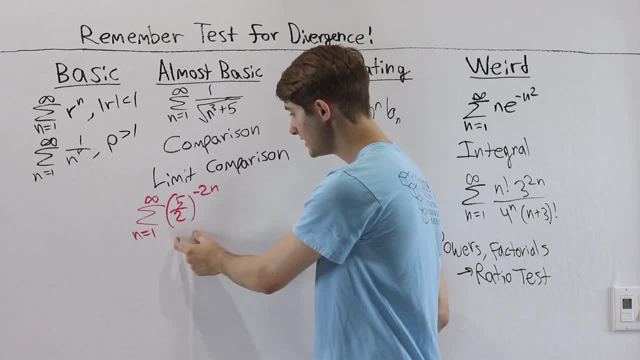 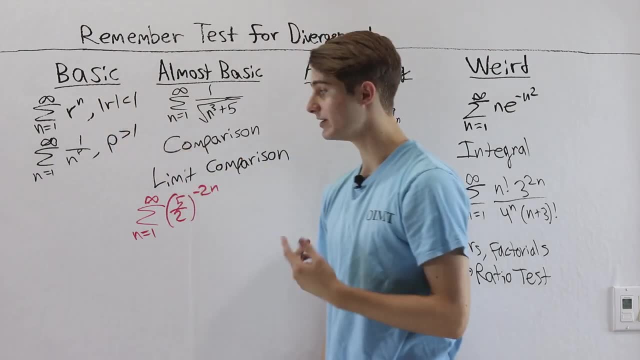 looks like a geometric series, right. So we have something and it's sort of to the power of n. So before we look at anything else, let's see if we can interpret it as just this basic form of a geometric series. To do that, we want to take a look at the exponent first, because we know that if we 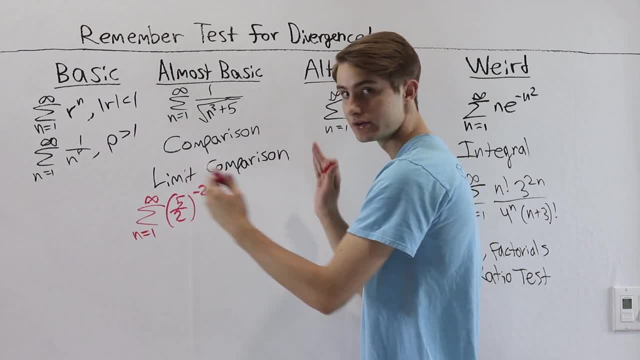 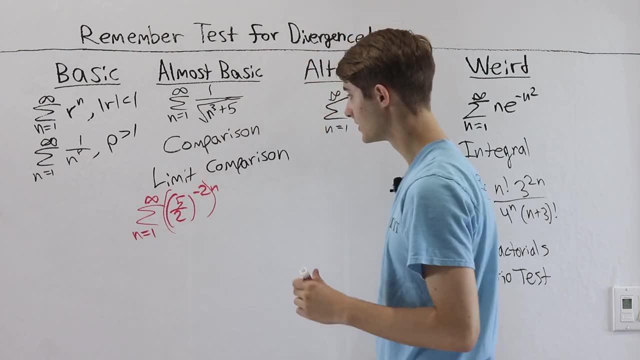 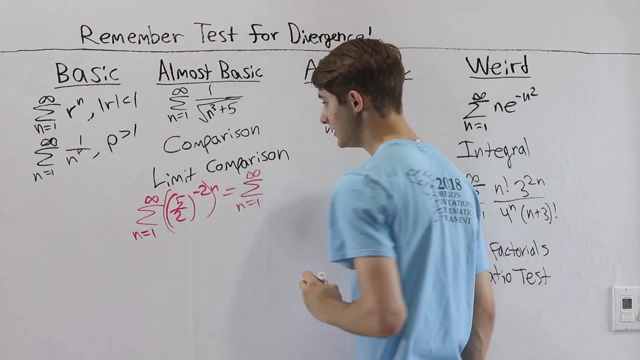 have five halves to the negative two, n. we can actually split up the powers As five halves to the power of negative two and then to the power of n, And once we do this we can rewrite the series in a form that we like a lot more. We'll have: the sum from n equals one to infinity. Well, what's five? 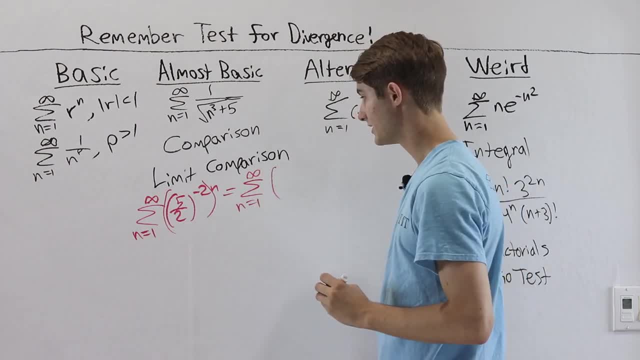 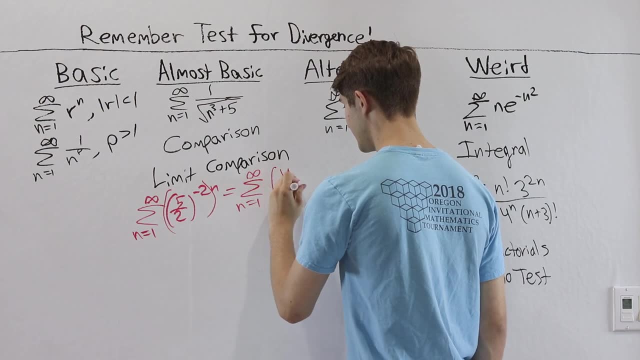 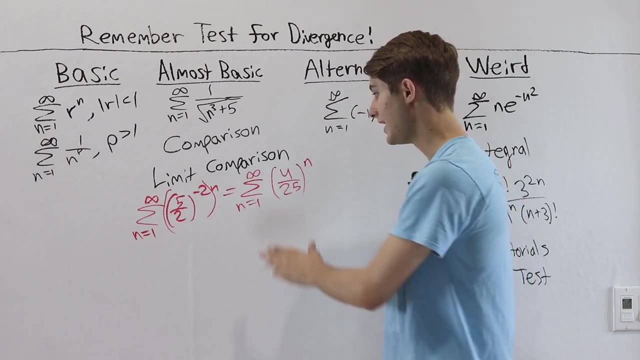 halves to the negative two. That's going to be the same thing as two fifths squared right. We have to flip it over for a negative power. That's going to be four divided by twenty, five right, Two squared over five squared, And we raise that to the power of n. And now this is exactly in the form of a geometric series: R to the n. 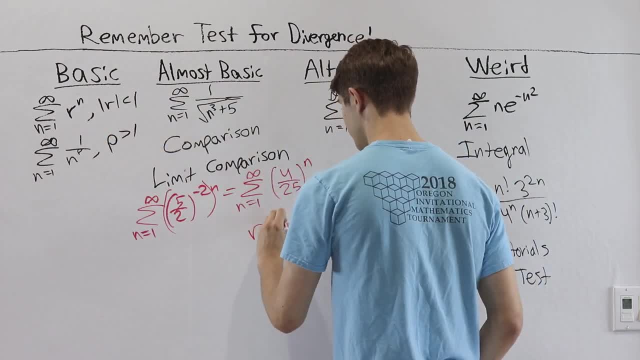 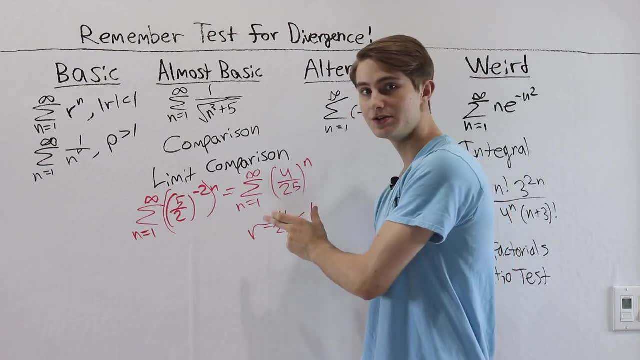 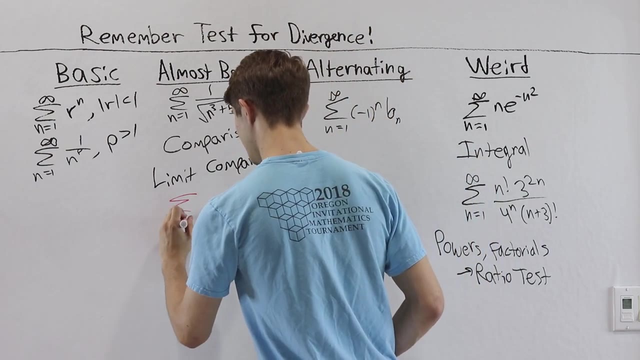 And our r is four over twenty five. So if we have our ratio being four twenty fifths, that's less than one, Which means we have proved that this series converges by the geometric series Next up. let's take a look at the sum from: n equals one to infinity, of n squared times three to the n. 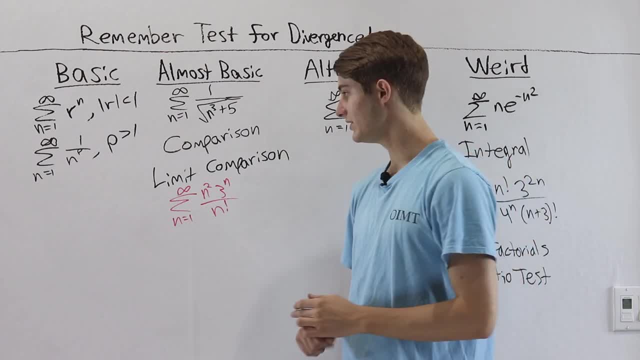 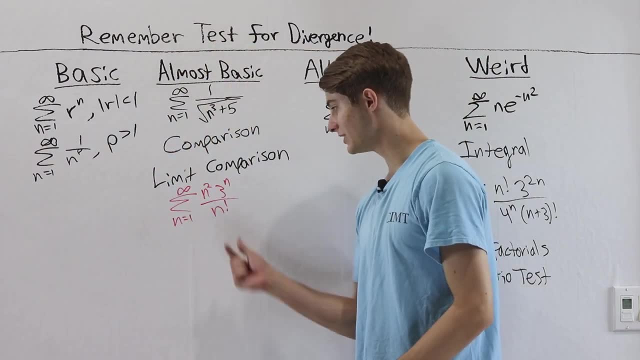 over n squared Notice in this case. this is already looking kind of weird. So we might be looking at this weird category to start out. And we also notice that we have factorials and we have numbers raised to the power of n And those two things. 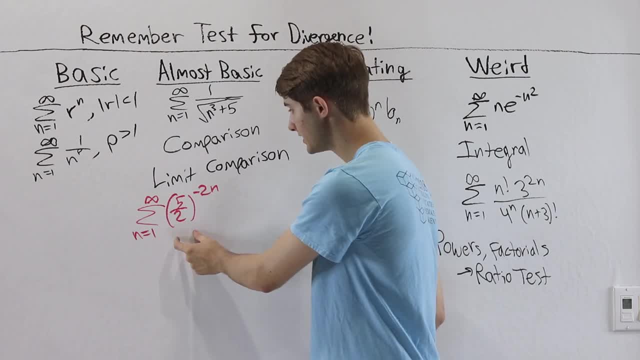 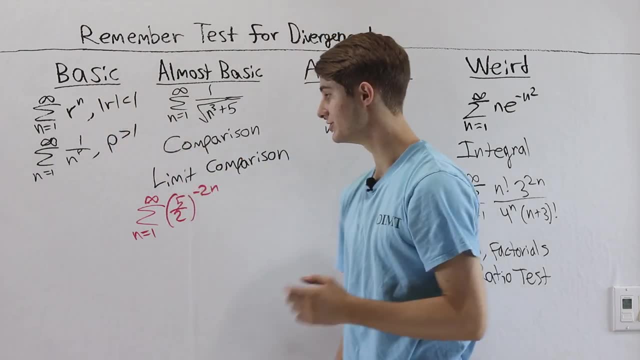 like a geometric series, right? So we have something and it's sort of to the power of n. So before we look at anything else, let's see if we can interpret it as just this basic form of a geometric series. To do that, we want to take a look at the. 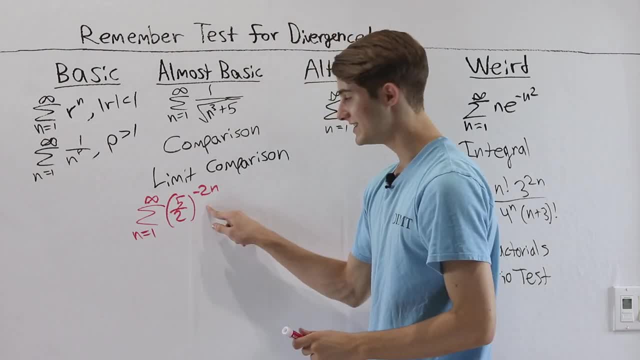 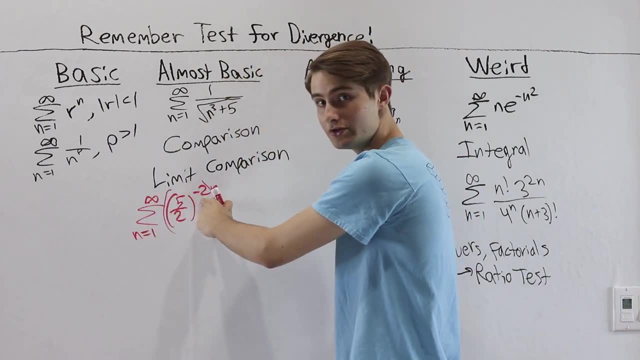 exponent. first, because we know that if we have 5 halves to the negative 2n, we can actually split up the powers as 5 halves to the power of negative 2 and then to the power of n, And once we do this we 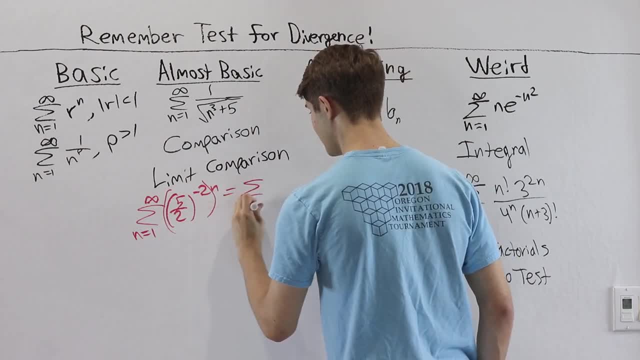 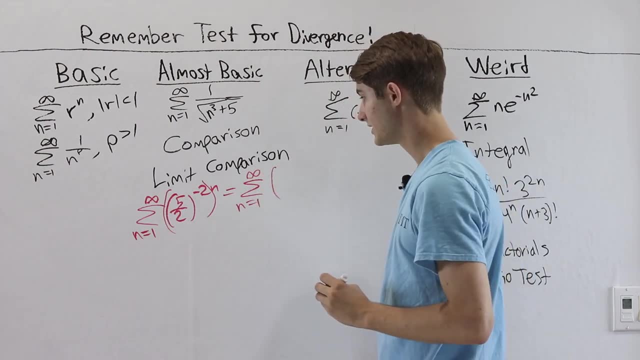 can rewrite the series in a form that we like a lot more. We'll have the sum from n equals 1 to infinity. Well, what's 5 halves to the negative 2?? That's going to be the same thing as 2 fifths squared right. We have to flip it over for a. 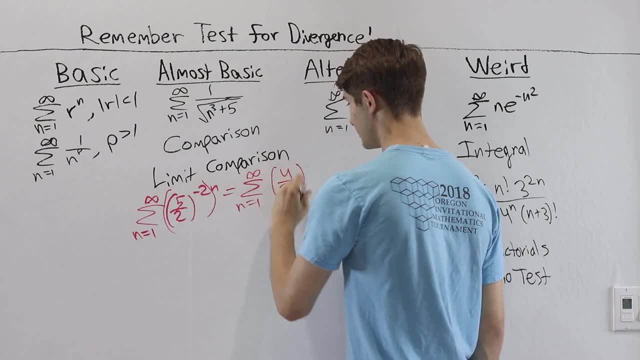 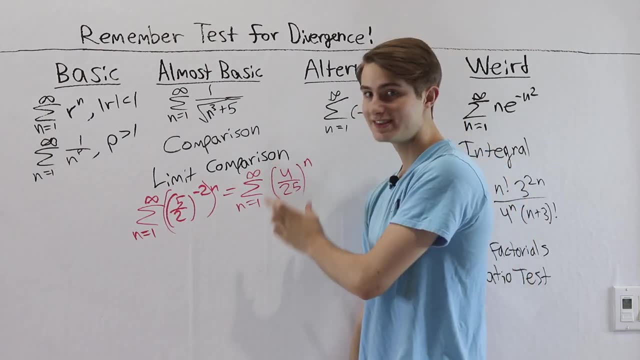 negative power, That's going to be 4 divided by 25, right, 2 squared over 5 squared, And then we raise that to the power of n. And now this is exactly in the form of a geometric series: r to the n, And our r is: 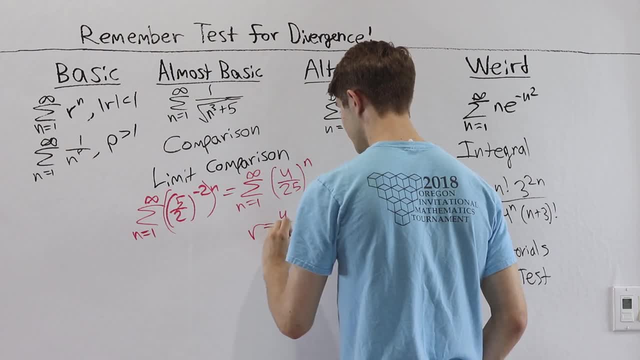 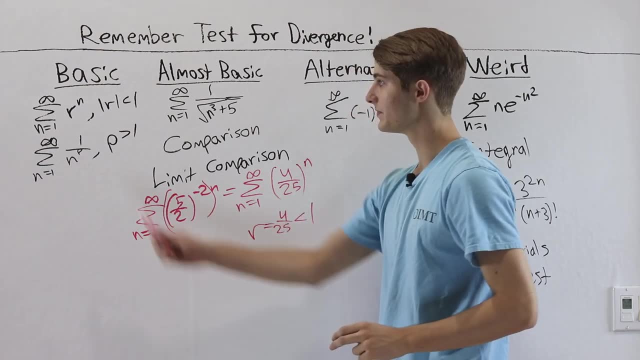 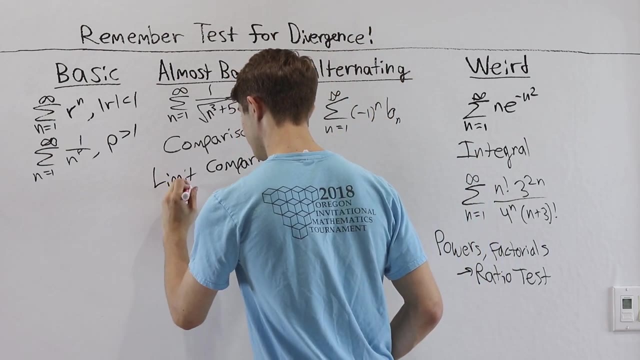 4 over 25.. So if we have our ratio being 4 twenty-fifths, that's less than 1, which means we have proved that this series converges by the geometric series Next up. let's take a look at the sum from n equals 1 to. 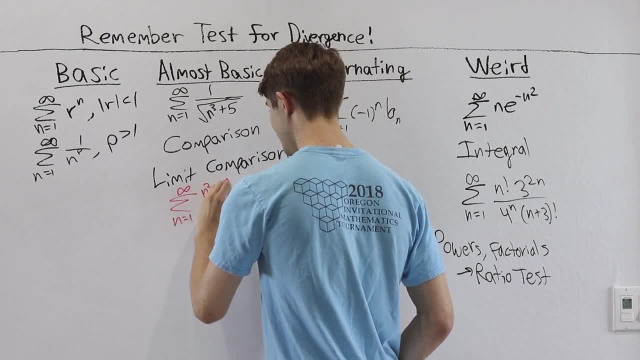 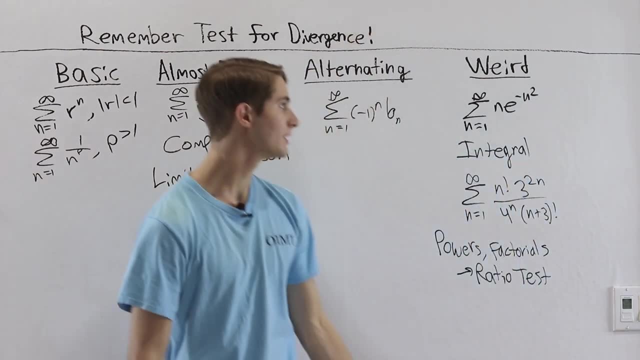 infinity of n squared times 3 to the n over n factorial. Notice, in this case this is already looking kind of weird. So we might be looking at this weird category to start out And we also notice that we have factorials and we have numbers. 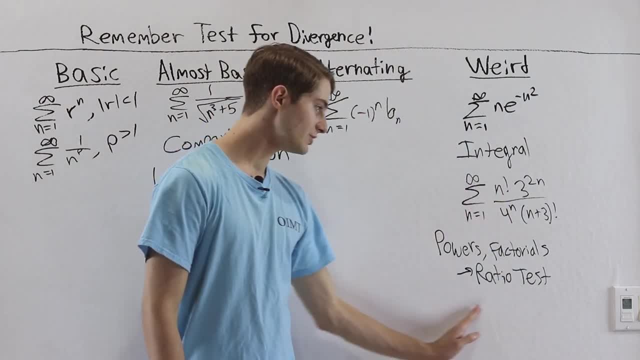 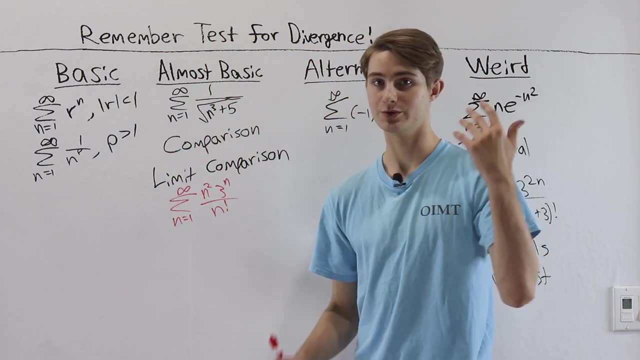 raised to the power of n, And those two things indicate to us that we should probably be using the ratio test. So in the case of this series, we won't go through all the work right now, because we're just trying to identify which test. 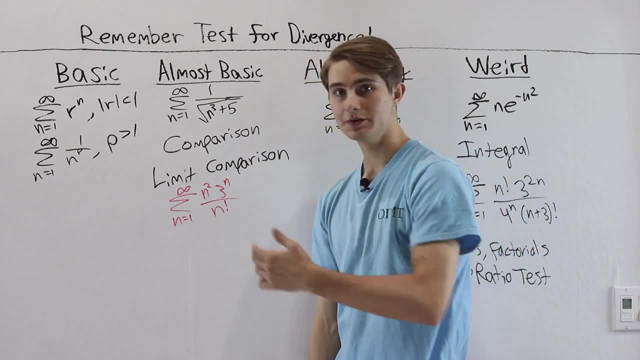 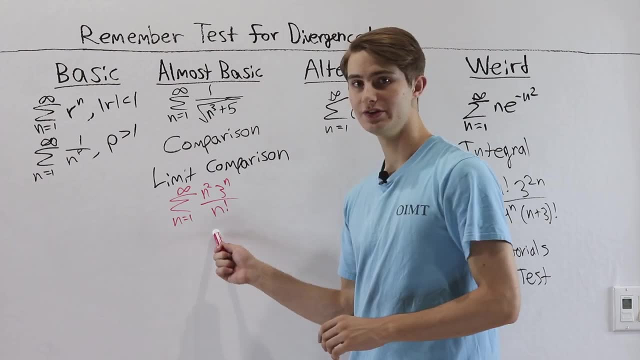 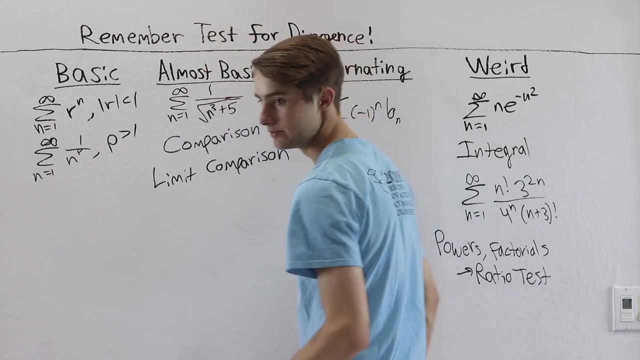 to use, But if we use the ratio test on this, we would be able to prove that the common ratio as n approaches infinity is less than 1, and therefore that this series converges by the ratio test. The next one we're going to take a look at will be a little different. It'll be this: 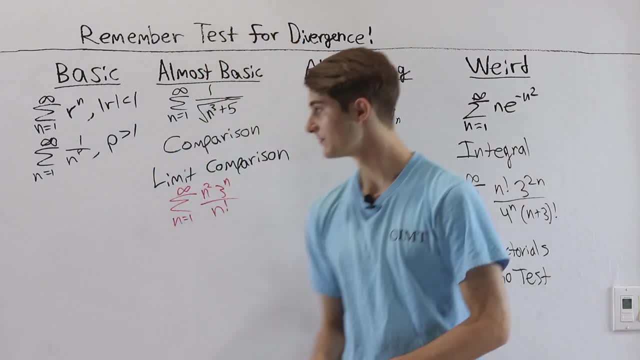 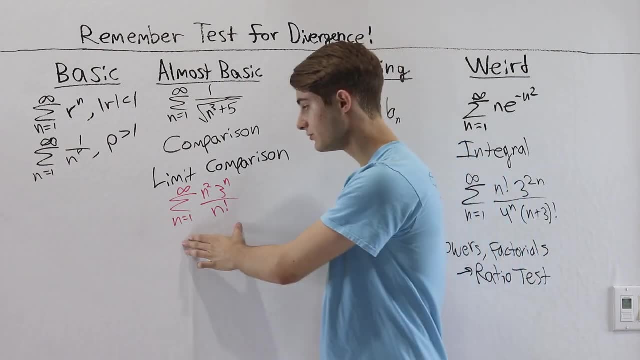 indicate to us that we should probably be using the ratio test. So in the case of this series, we won't go through all the work right now, because we're just trying to identify which test to use. But if we use the ratio test, on this we 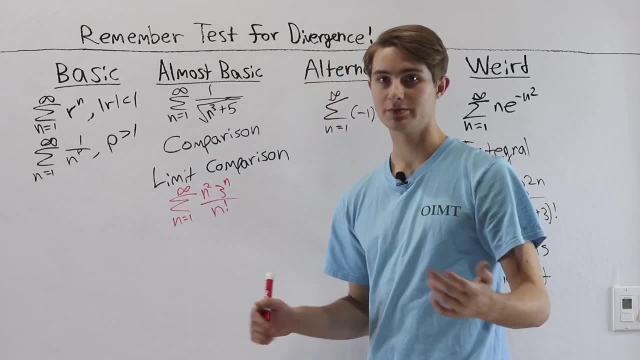 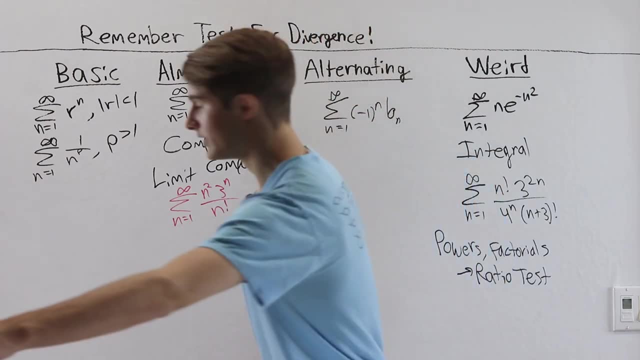 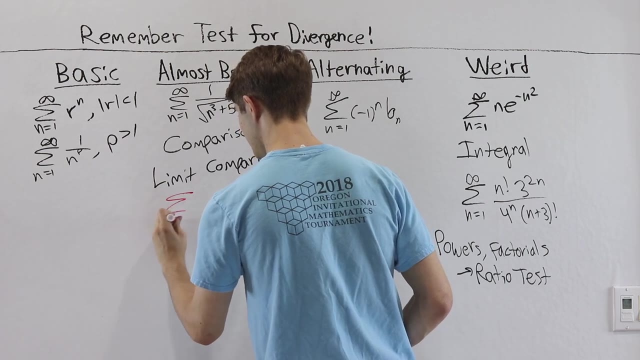 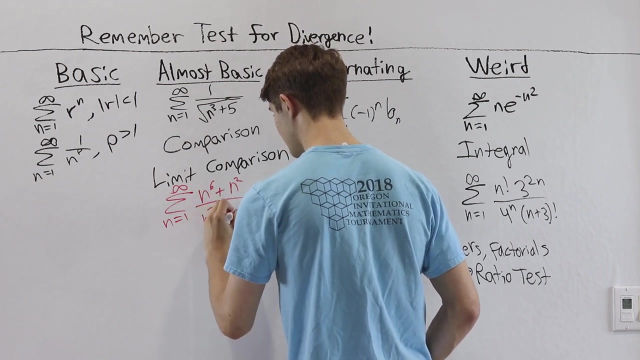 would be able to prove that the Common ratio is n approaches infinity, is less than one, and therefore that this series converges by the ratio test. The next one we're going to take a look at Will be a little different. It'll be the sum from n equals one to infinity, of n to the sixth plus n, squared over n to the seventh plus three. 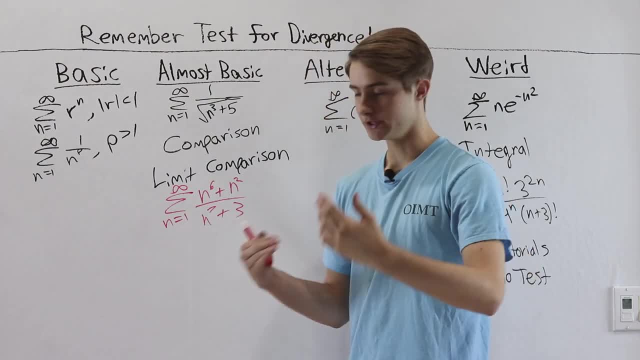 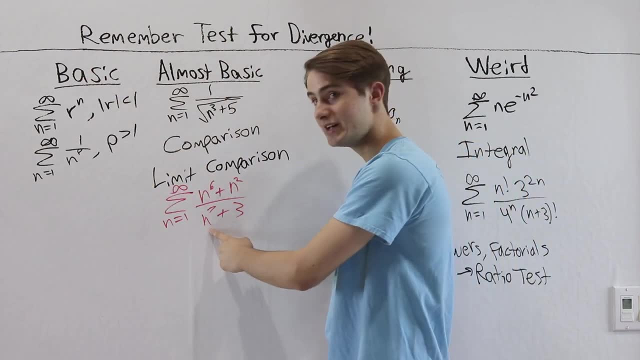 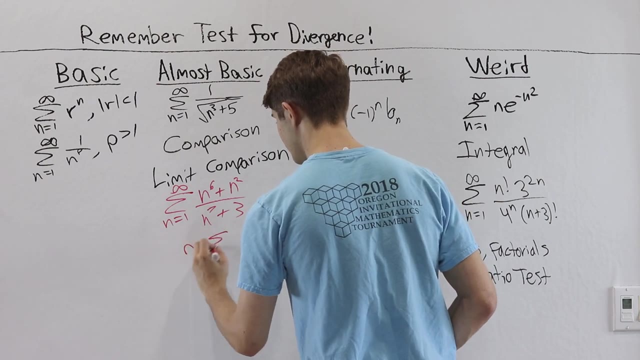 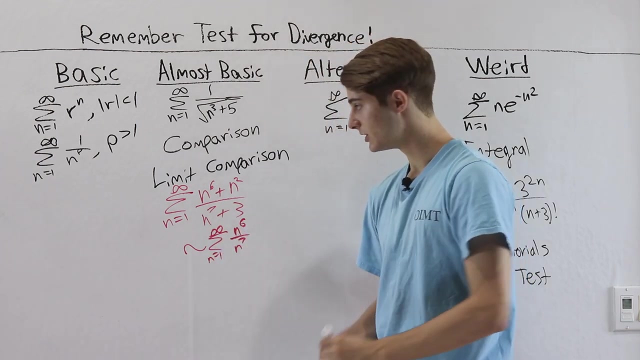 Now notice, in this case, as n gets really really large, N to the sixth is going to be much, much, much bigger than n squared, and n to the seventh is going to be much, much bigger than three, Which means that really, what we're looking at is very similar to the sum from n equals one to infinity, of n to the sixth over n to the seventh. 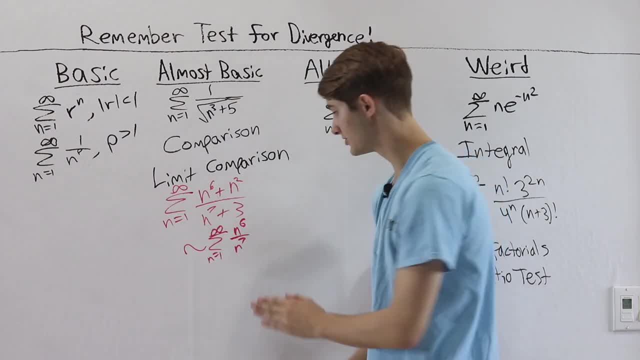 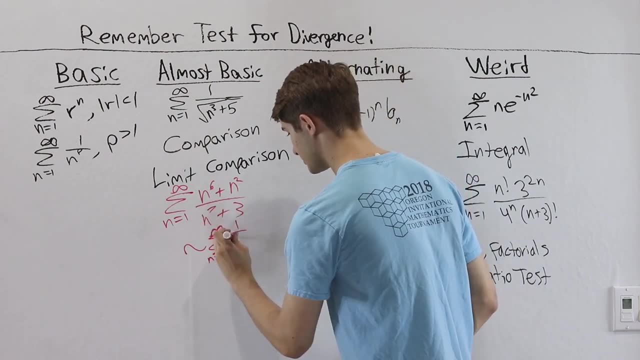 But we can write this n to the sixth over n to the seventh. We put the powers together as just one over n. So we can say that our series that we have here Is very much Like one over n, as n gets very large. 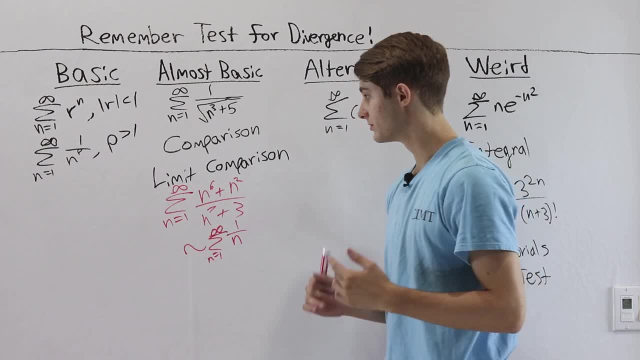 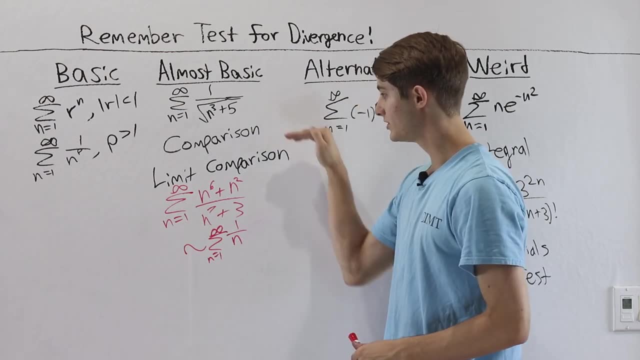 And this is a type of p series. So in reality, the series that we're looking at here is an instance of an almost basic series. So we're going to want to use either the comparison test or the limit comparison test to turn what we have here into the p series. 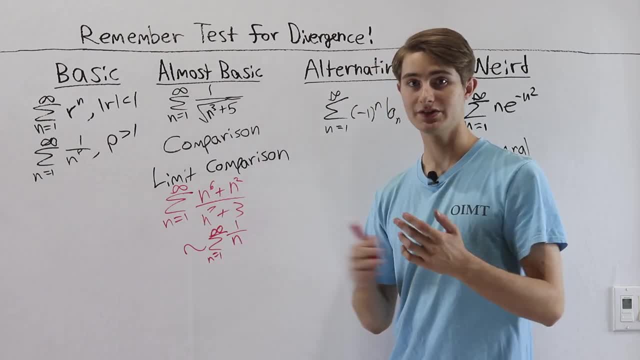 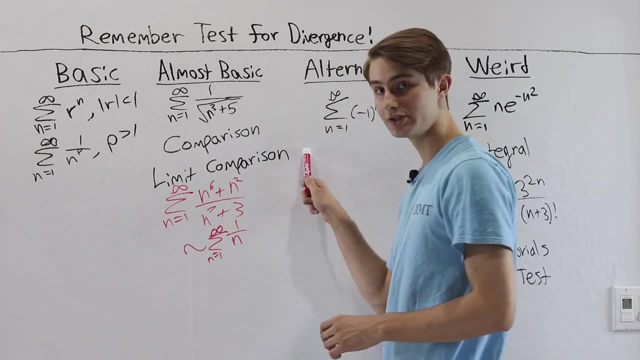 Now, because we have this n squared on the top, using the comparison test is going to be a little strange, So I think it would be easier in this instance To use the limit comparison test. So we would use the limit comparison test to compare this series to the sum of one over n. 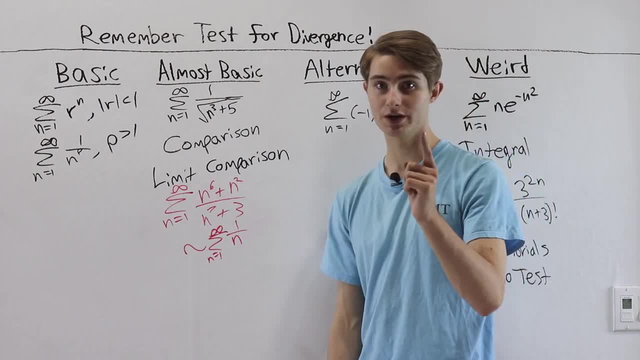 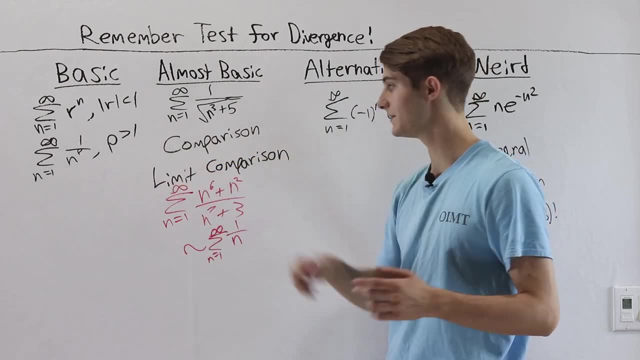 And then we would get the value of one as our answer. And because one is the result that we get and the sum of one over n diverges, the harmonic series p is less than or equal to one, Then we know that our original series diverges as well. 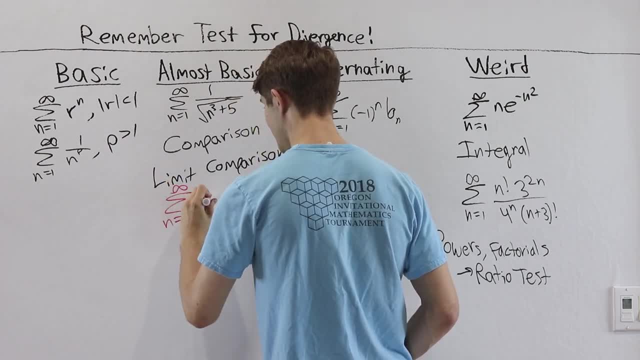 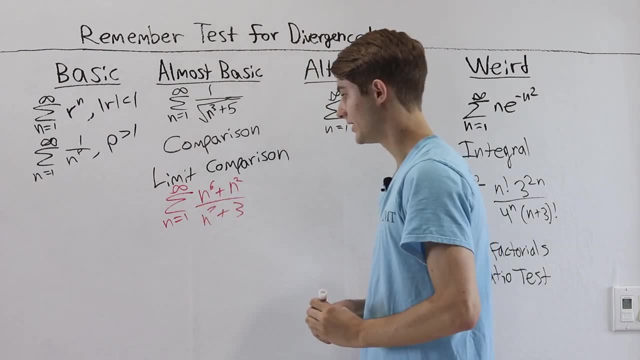 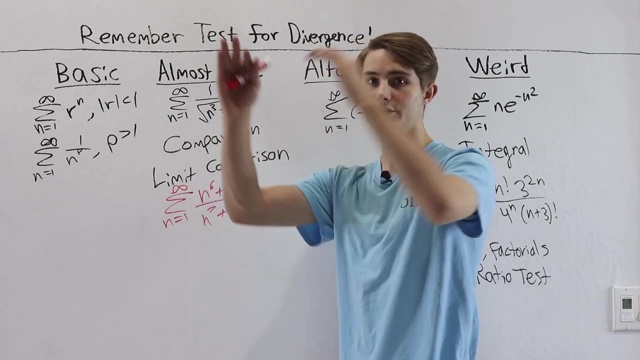 sum from n equals 1 to infinity, of n to the 6th plus n, squared over n to the 7th plus 3.. Now Notice, in this case, as n gets really really large, n to the 6th is going to be much, much, much bigger than n squared. 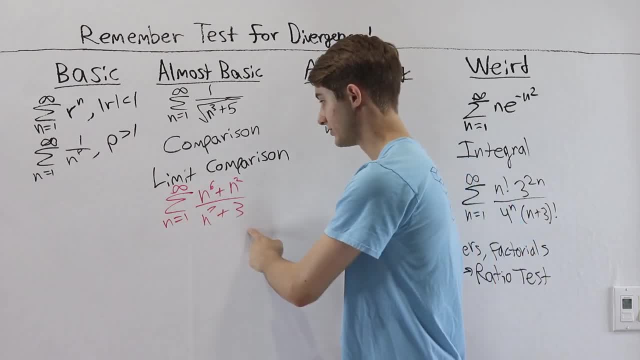 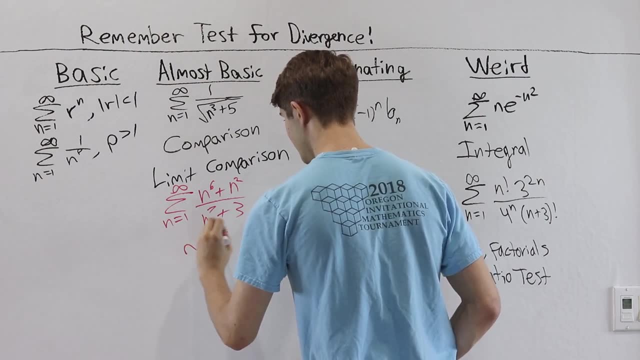 and n to the 7th is going to be much, much bigger than 3, which means that, really, what we're looking at is very similar to the sum from n equals 1 to infinity, of n to the 6th over n to the 7th. 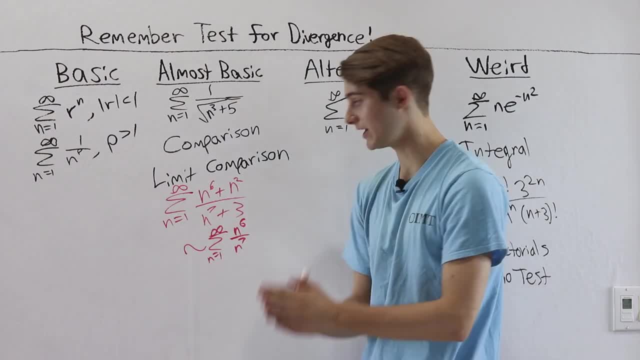 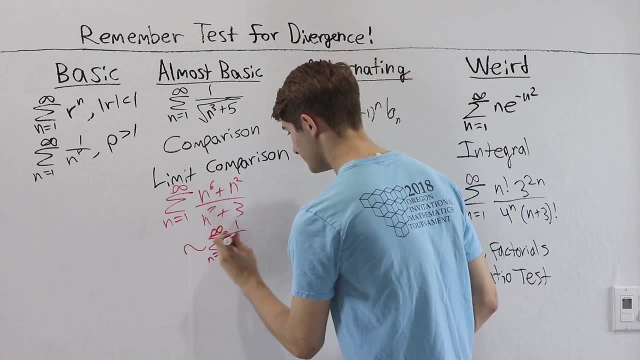 But we can write this n to the 6th over n to the 7th. we put the powers together as just 1 over n. So we can say that our series that we have here is very much like 1 over n, as n gets very large. 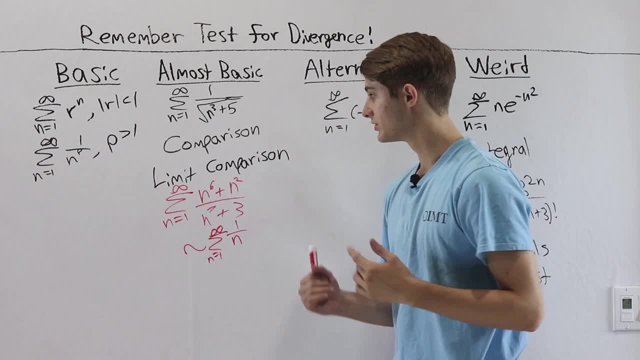 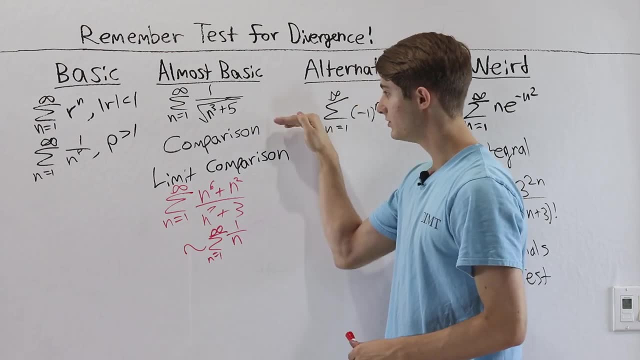 And this is a type of p-series. So in reality, the series that we're looking at here is an instance of an almost basic series. So we're going to want to use either the comparison test or the limit comparison test to turn what we have here into the p-series. 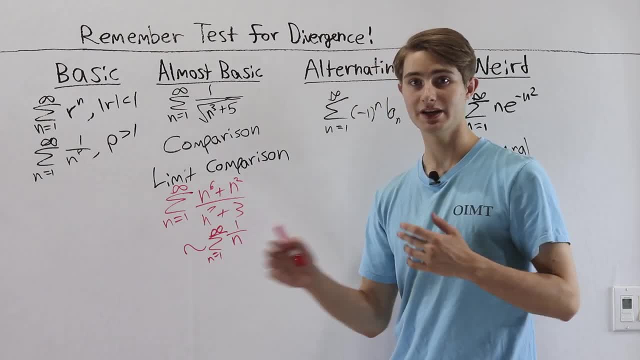 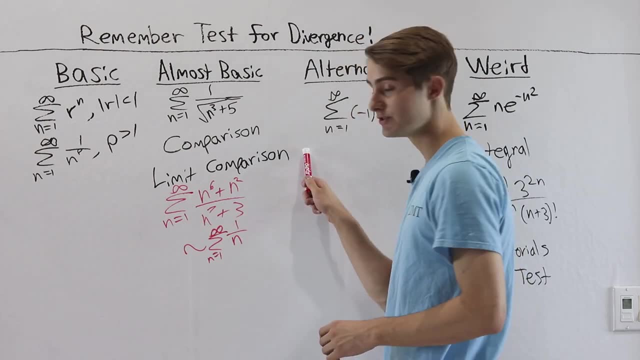 Now, because we have this n squared on the top, using the comparison test is going to be a little strange, So I think it would be easier in this instance to use the limit comparison test. So we would use the limit comparison test to compare this series to the sum of 1 over n. 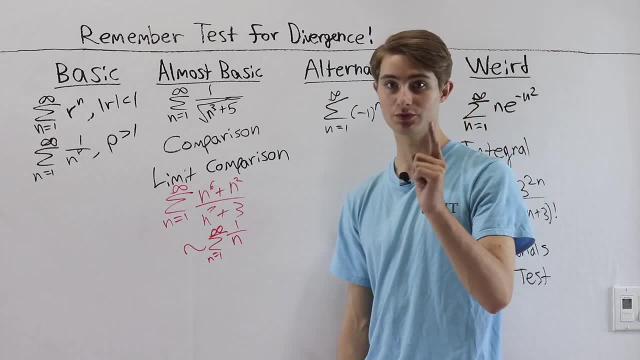 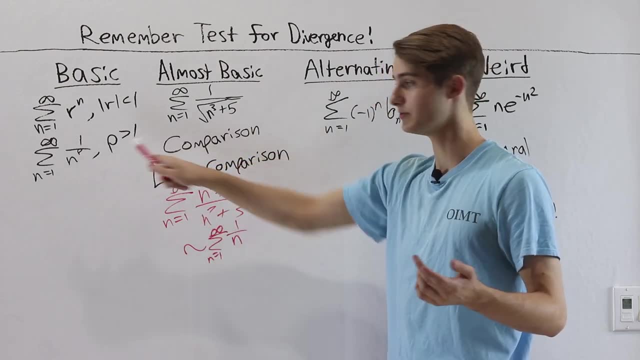 And then we would get the value of 1 as our answer. And because 1 is the result that we get and the sum of 1 over n diverges, the harmonic series p is less than or equal to 1, then we know that our original series diverges as well. 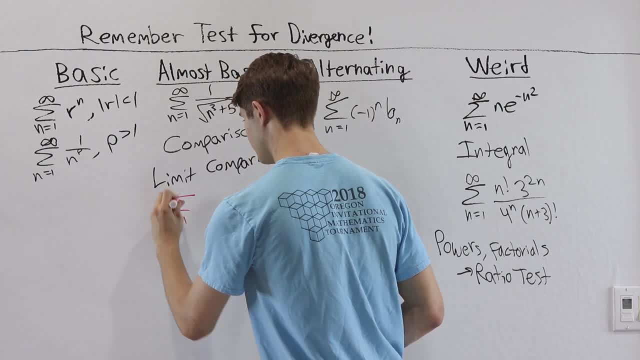 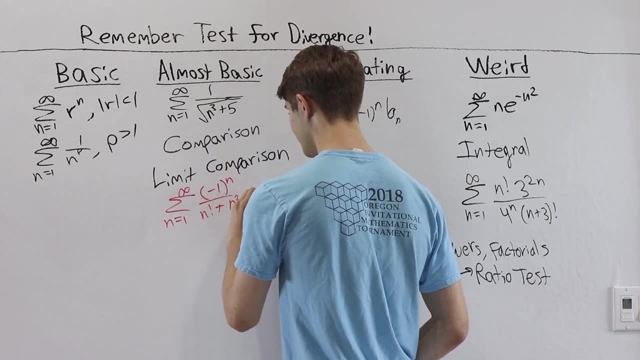 Next up, let's take a look at the sum from n equals 1 to infinity, of negative 1 to the n over n factorial plus n squared plus 3.. Now, you might be tempted to look at this as a weird series. 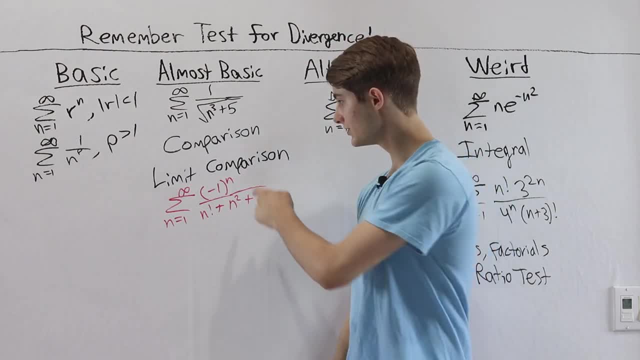 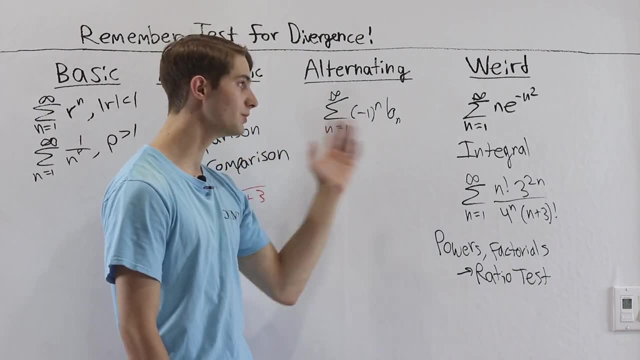 because of the n- factorial, and that might work. But also notice that we have a negative 1 to the n in the numerator here, which means this is an alternating series. The first thing we always want to try is the alternating series test. 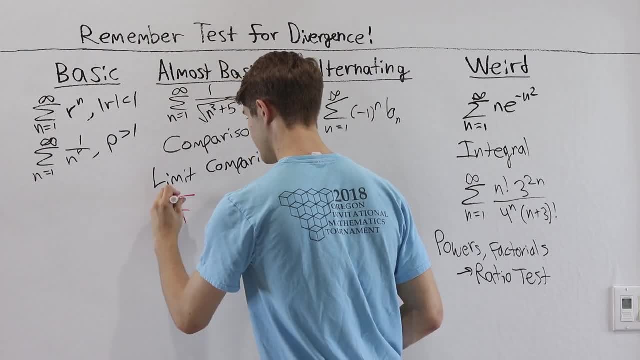 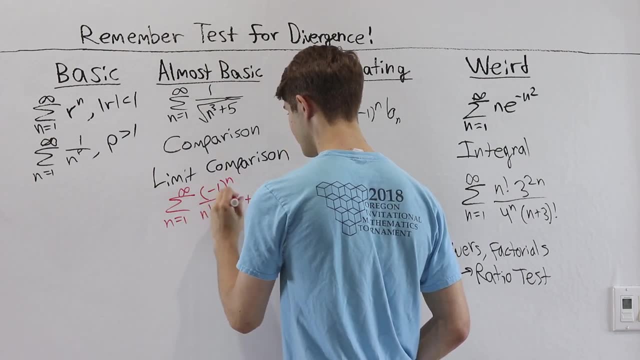 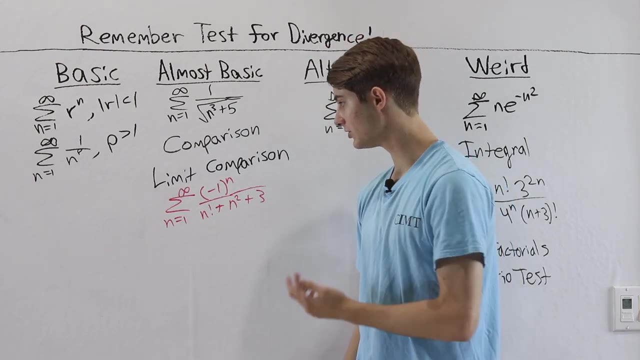 Next up, let's take a look at the sum from n equals one to infinity, of negative one To The n over n factorial, plus n squared plus three. Now you might be tempted to look at this as a weird series because of the n? factorial, and that might work. 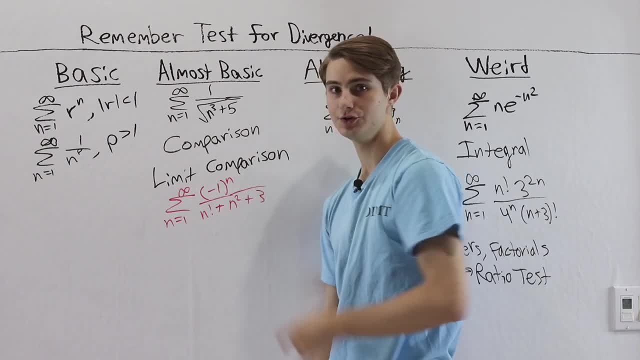 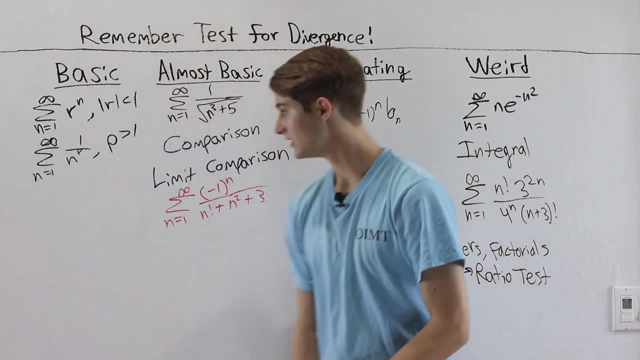 But also notice that we have a negative one to the n in the numerator here, which means this is an alternating series. The first thing we always want to try is the alternating series test, And in this case we would actually be able to prove that this sum converges by the alternating series test. 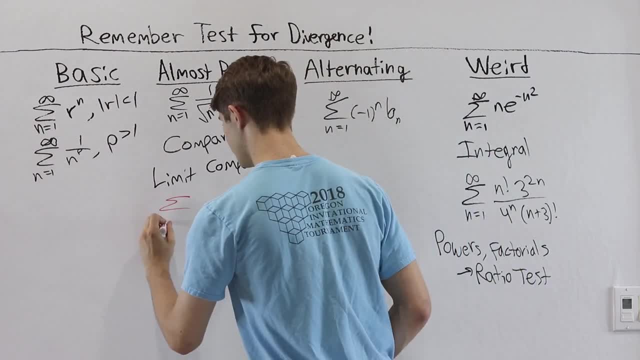 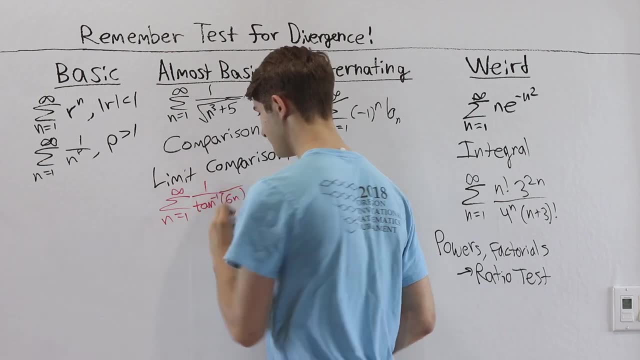 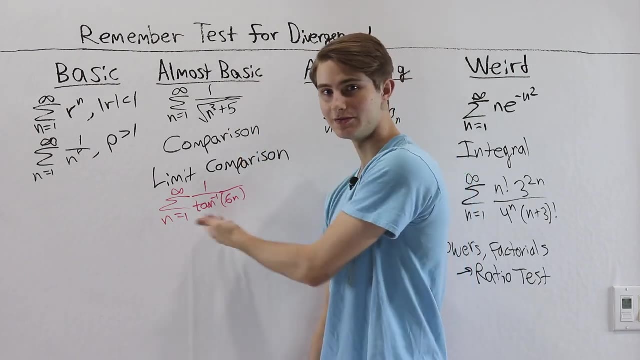 So we're going to look at one More series here, which is: the sum from n equals one to infinity of one over the inverse tangent of six. and Now this is not a basic series, it's not almost basic either, because we have this inverse trig function. that's kind of strange, it's not alternating. 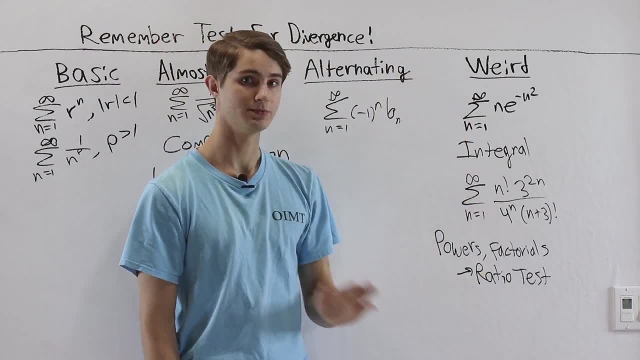 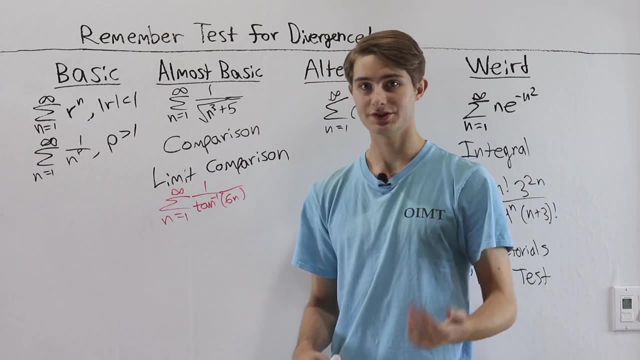 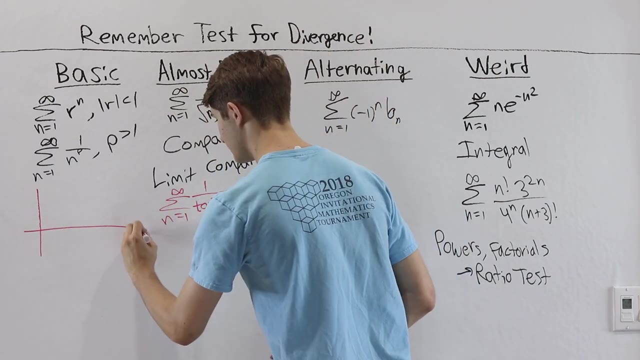 And we might be tempted to look at this as a weird series, but we should hold on first and examine what this series actually looks like. If we think about the inverse tangent function, What would the graph of that function look like? Well as n. 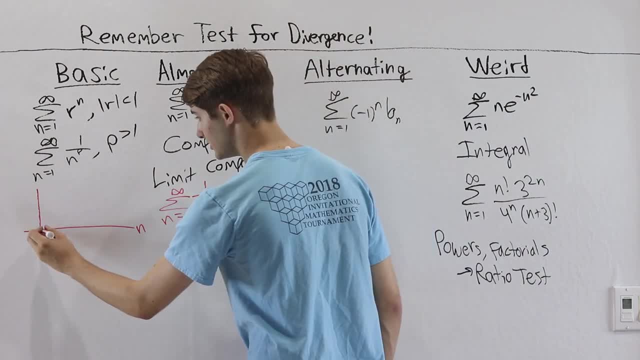 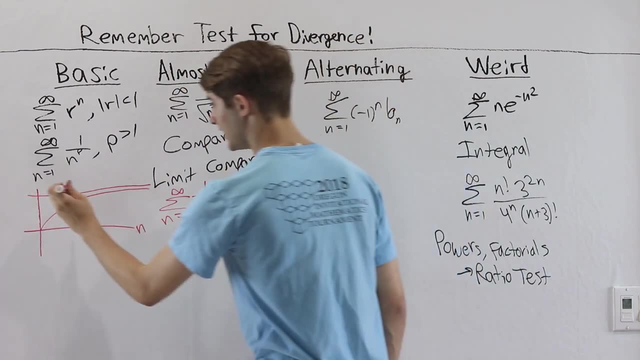 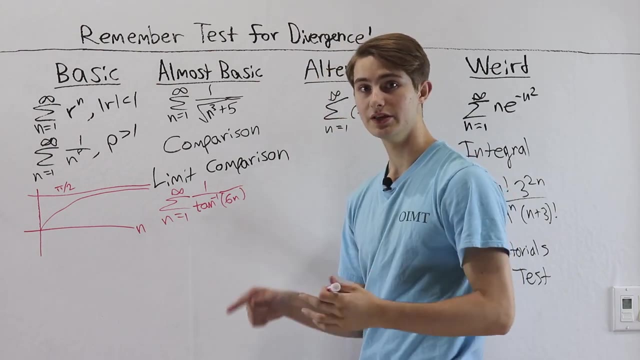 On this x axis here increases. the inverse tangent is going to look like this: It's going to have a vertical asymptote At the value of pi over two, Which means if we divide By the inverse tangent, This is not going to go to zero. 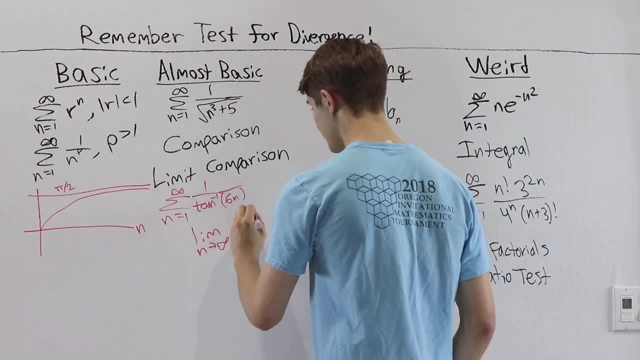 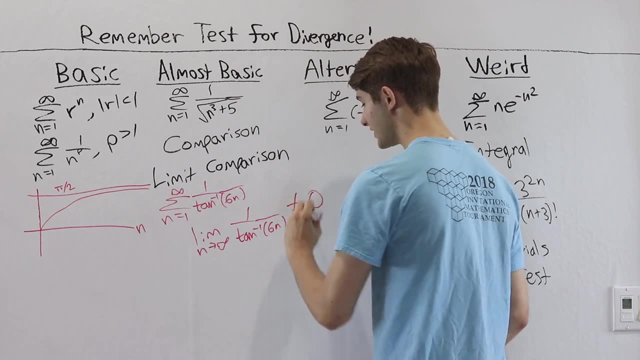 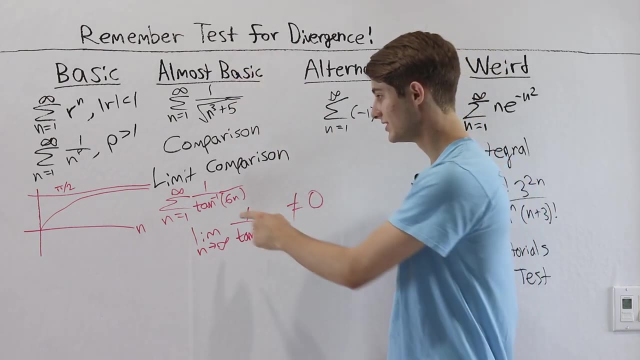 So if we take the limit As n approaches infinity, Of the inside of the sum one over the inverse tangent Of six, and That result is not going to be zero, And if this limit is not equal to zero, Then by the test for divergence. 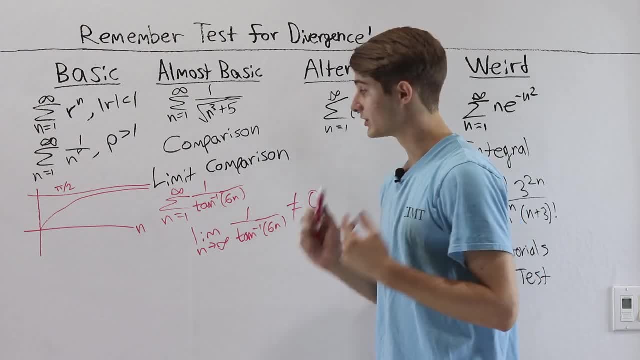 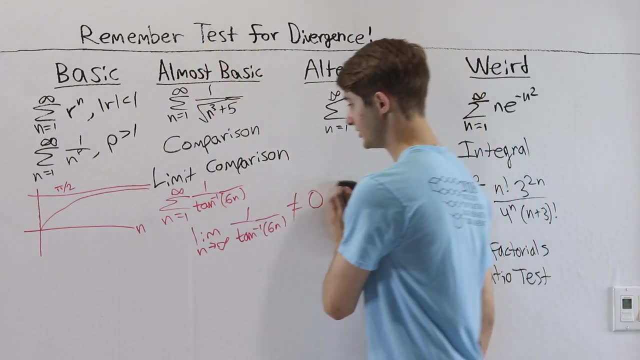 This series must diverge. So this exercise is a quick reminder that any time we're doing serious, no matter what it looks like, we always have to remember the test for divergence, Because it might seem that It would be a good idea To try some other series. 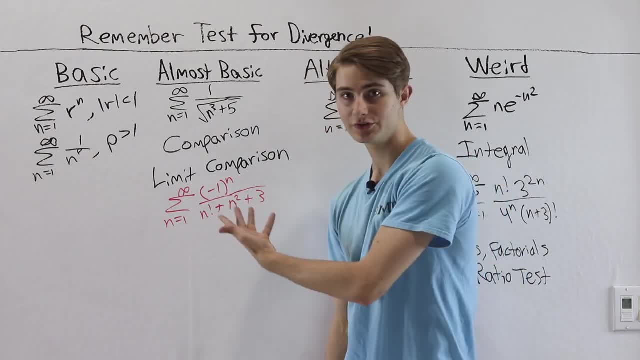 And in this case we would actually be able to prove that this sum converges to the n squared plus 3.. So we would be able to prove that this sum converges to the n squared plus 3.. So we would be able to prove that this sum converges to the n squared plus 3.. 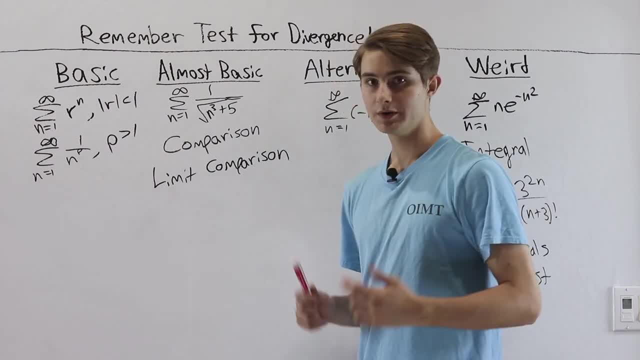 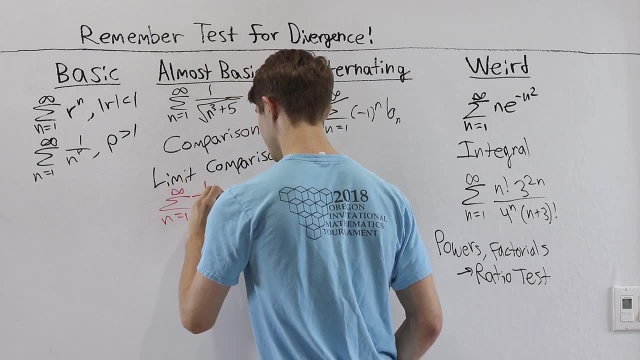 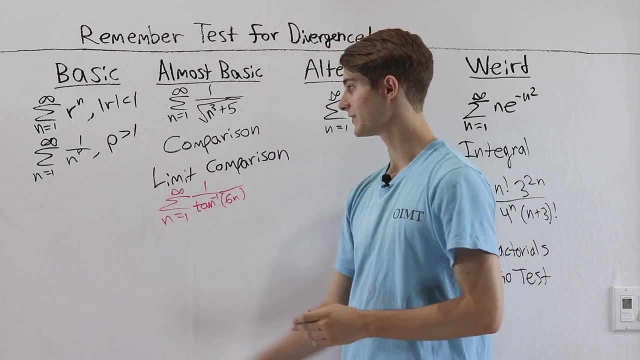 by the alternating series test. So we're going to look at one more series here, which is the sum from n equals 1 to infinity of 1 over the inverse tangent of 6n. Now this is not a basic series. It's not almost basic either. 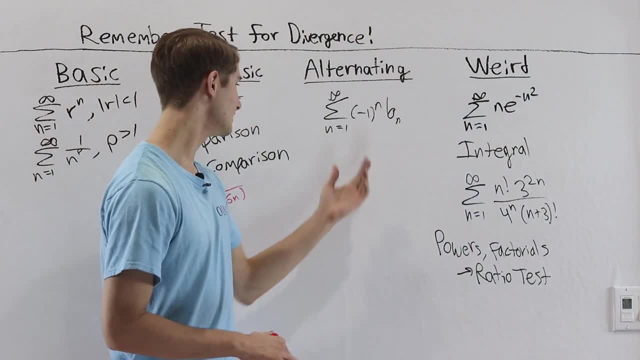 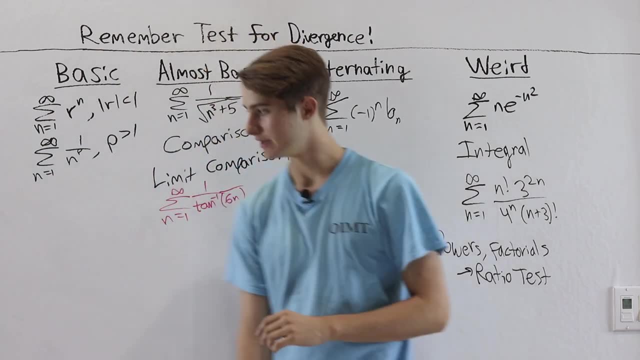 because we have this inverse trig function. That's kind of strange. It's not alternating And we might be tempted to look at this as a weird series. But we should hold on first And examine what this series actually looks like If we think about the inverse tangent function. 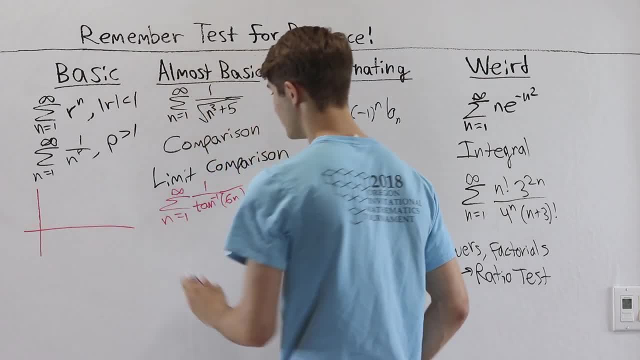 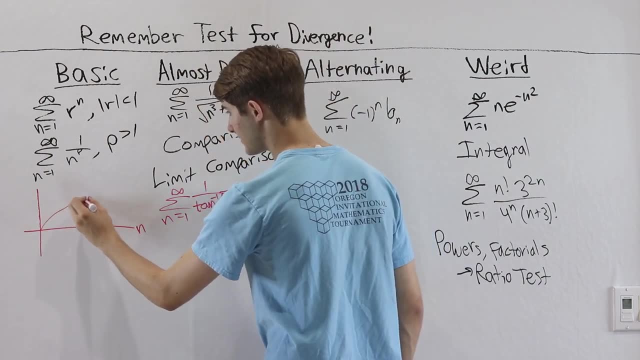 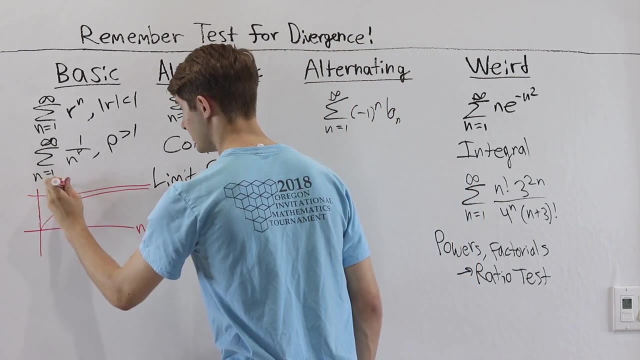 what would the graph of that function look like? Well, as n on this x-axis here increases, the inverse tangent is going to look like this: It's going to have a vertical asymptote at the value of pi over 2, which means, if we divide by the inverse tangent, 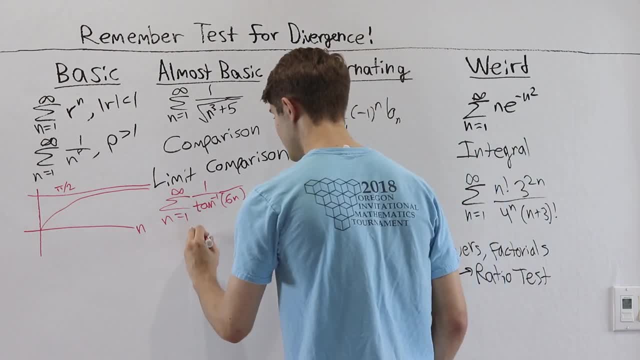 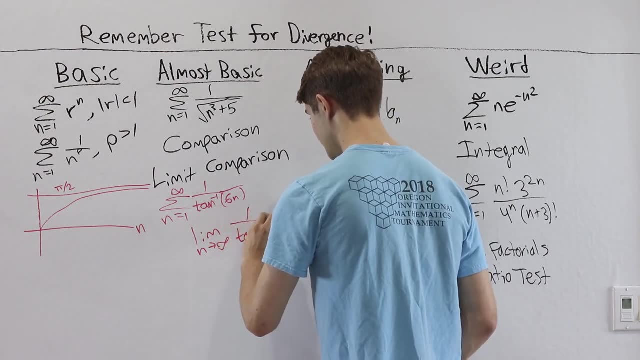 this is not going to go to 0. So if we take the limit as n approaches infinity of the inside of this sum, 1 over the inverse tangent of 6n, that result is not going to be 0. And if this limit is not equal to 0,. 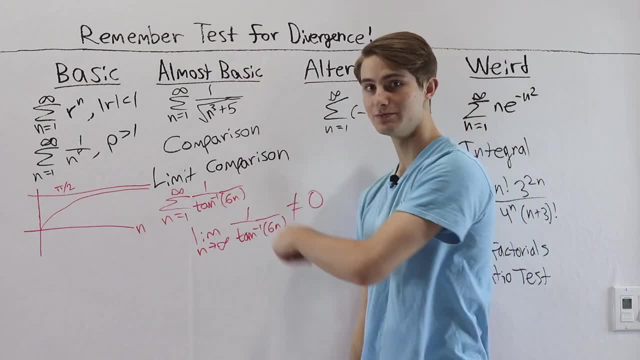 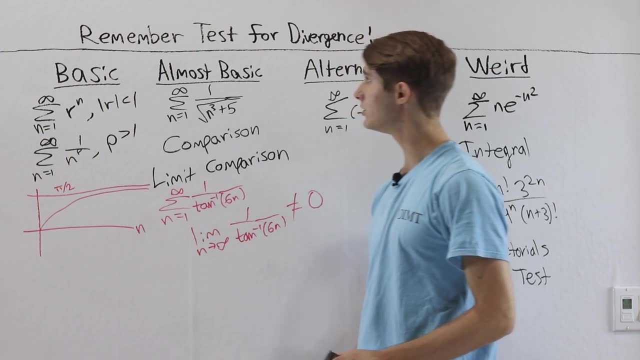 then by the test for divergence, this series must diverge. So this exercise is a quick reminder that any time we're doing series, no matter what it looks like, we always have to remember the test for divergence Because it might seem that it would be a good idea. 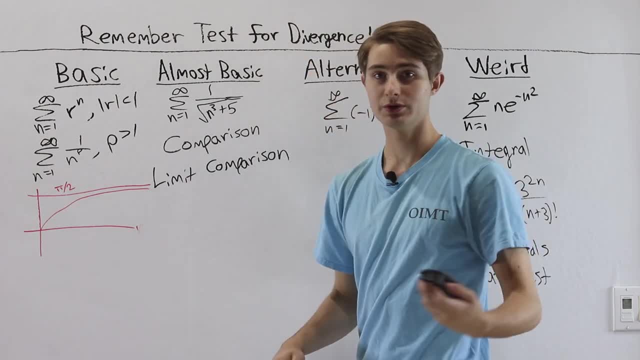 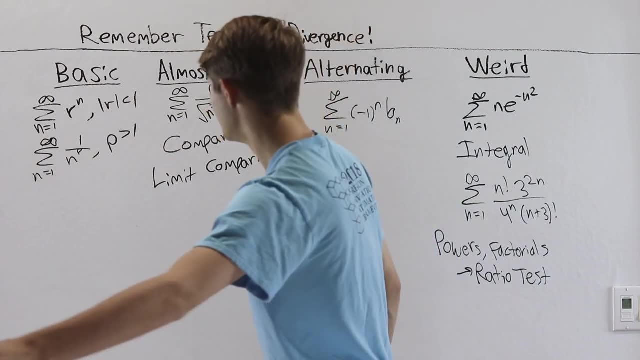 to try some other series test. but as long as we can prove that the inside of the sum never goes to 0, we can get off really easy, just doing a limit and proving that it diverges. So these are the four categories that it's always good to remember. 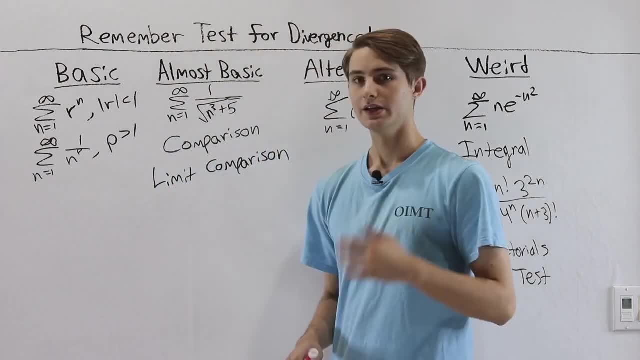 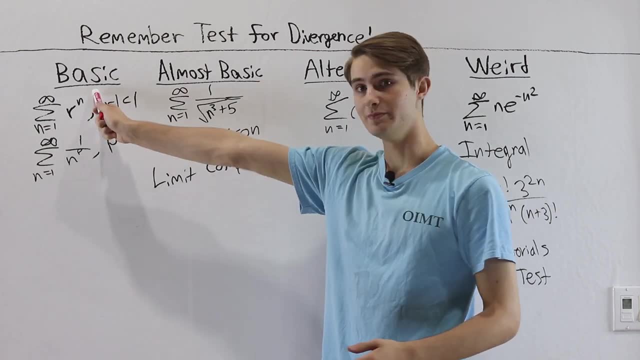 when you're trying to figure out which convergence test to use, If you see a sum that you can write in the form of some number to the power of n, and that's a geometric series. so that's a basic form that you can evaluate directly.